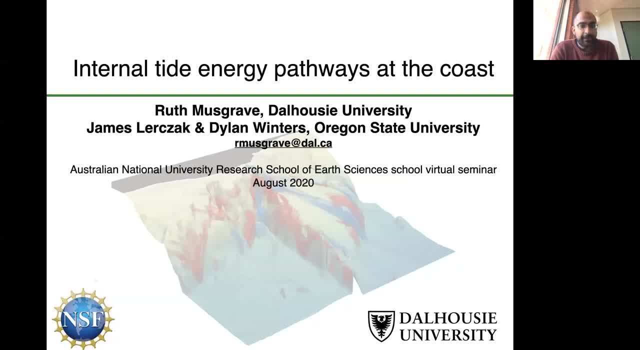 Hi there, Okay, Hi, it's my privilege and honor to introduce Ruth Musgrave. So Ruth did her honors with Louise Morezzi at Monash And I guess after finishing her honors Louise convinced her that the right way forward is oceanography. Then she went to Scripps. 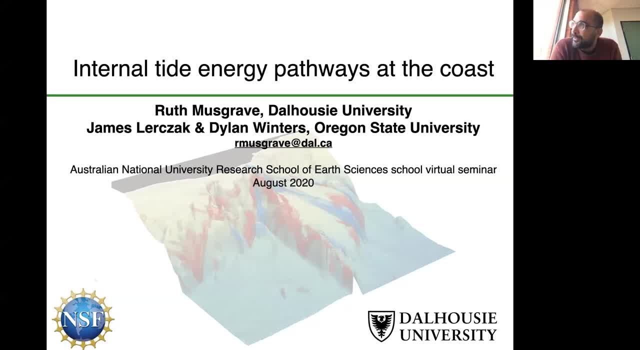 Institution of Oceanography at San Diego and she did her PhD there And she finished, I think, just a bit before I arrived there to do a postdoc. Then she went on for a postdoc at MIT Ocean Engineering School and afterwards at Woods School Oceanographic Institution. 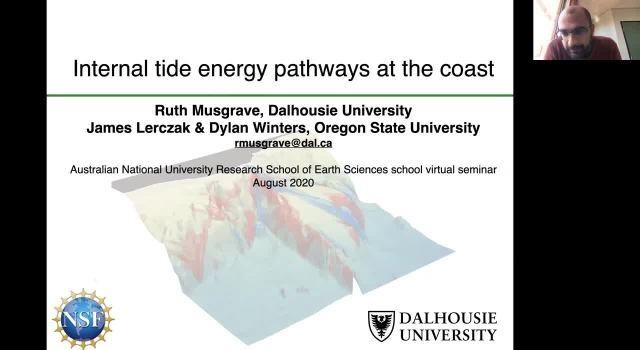 And recently, six months ago, eight months ago. how long have you been there? Almost a year, Almost a year. So, COVID, time flies. Recently she went to Canada, in Dalhousie, to start a faculty position. So, since it's already, 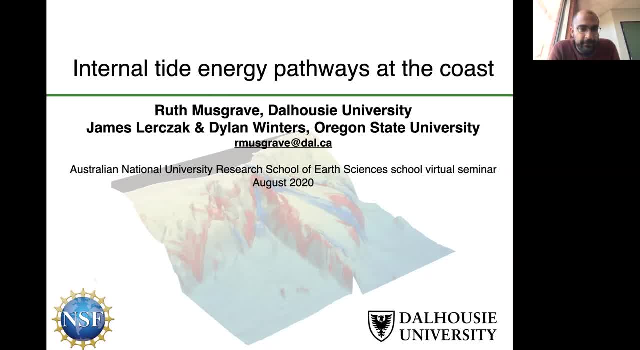 after midnight there. I'll hand over to you, And I want to make a note that tomorrow morning, 9 am Canberra time, I arranged a Zoom call with Ruth for anyone who wants to chat further on her research or on the talk or anything, so that we don't go up to 2 am in Canada tonight. Okay, 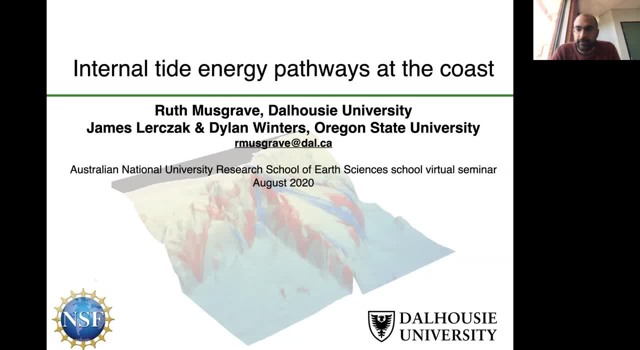 So I'll send out and Zoom details after the seminar. Yeah, thank you, And that includes the student catch up that we often do after the seminar. So we're going to spare Ruth that too, And so they can join tomorrow, if that's okay. 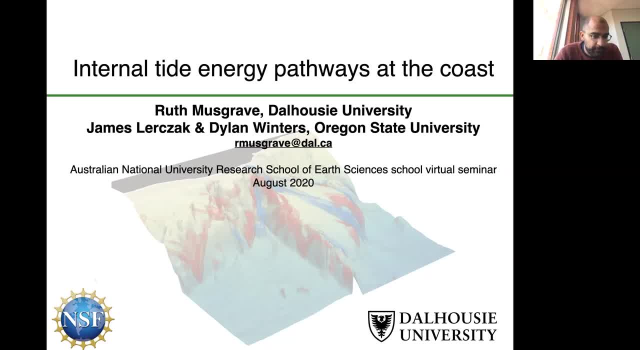 Yeah, sure, Okay, Off you go. The stage is yours. Well, thank you for the introduction And thank you to everyone for being here. I'm very happy to be able to present my research at ANU from the comfort of my own home. 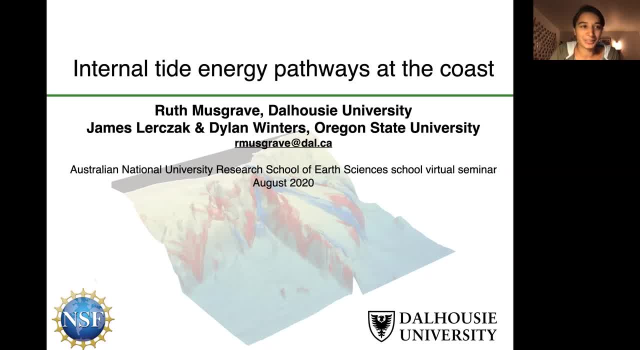 here in Canada. So I'm going to tell you today about some work that I've been doing recently with my collaborators, Jim Lursak and Dylan Winters at OSU- Oregon State University- And we've been thinking about internal tide energy pathways at the coast. 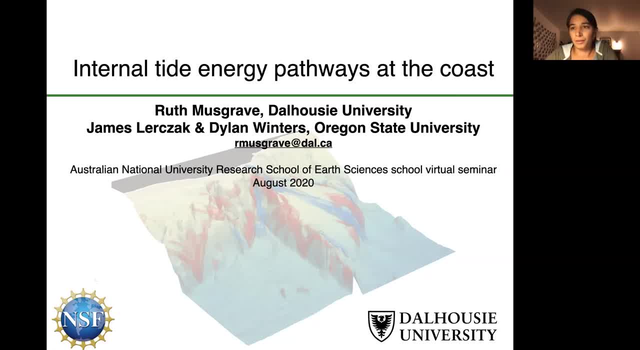 Advance that way. Okay, So a brief talk overview. I'm going to split the talk into three parts. I'm going to start with a really big picture view of ocean mixing and its role in climate, which kind of motivates all of this work. We still see the title slide, Is that right? 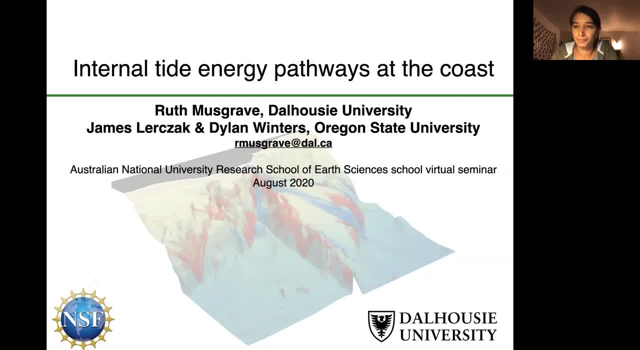 How about now? No, I still see this title. Yeah, still the title. That's interesting. Perhaps I'm sharing sharing. Actually, I have a button here that says resume share. Sharing is paused. That's what you need to do. Go for it. 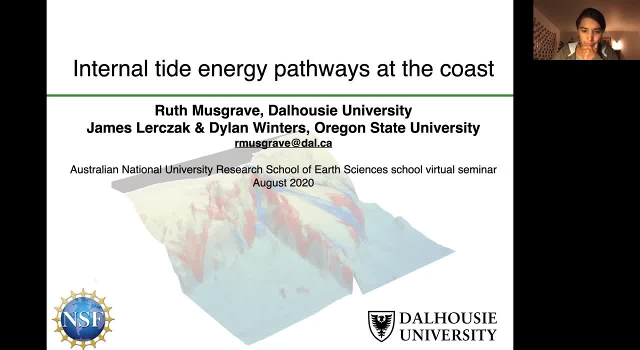 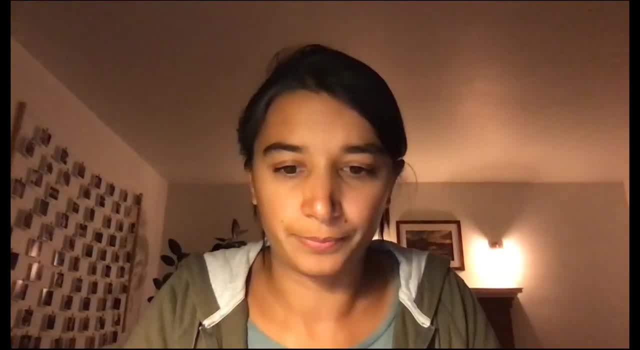 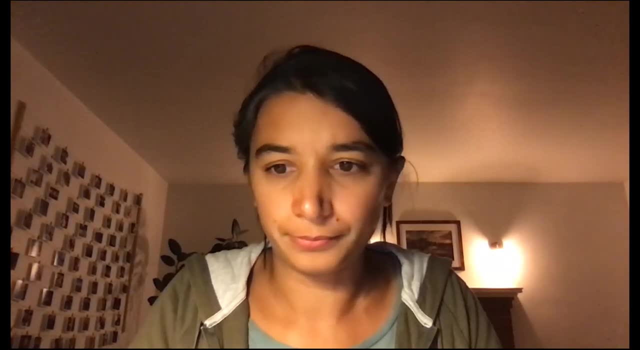 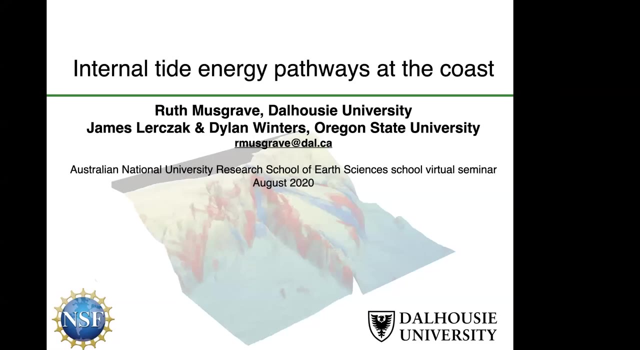 Well, I've gone for it. Has that made a difference? You might have to refresh the. Okay, I'm going to stop sharing and then I'm going to start again. Okay, Can you see my screen again? Yep, Okay, You see the next slide. 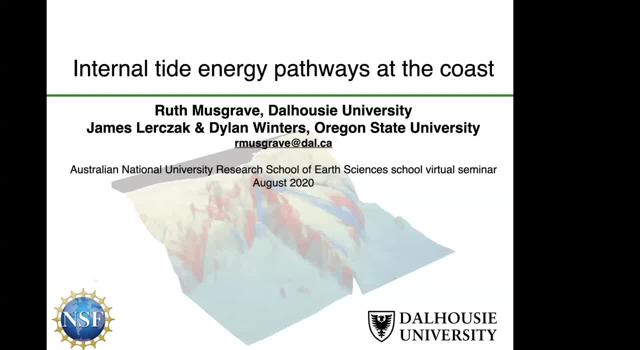 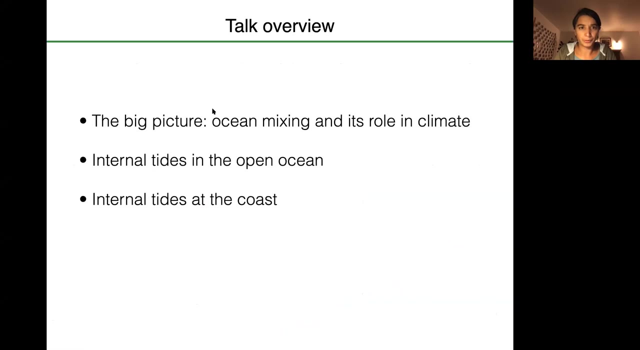 No, yeah, Sharing is paused. Bring your shared window to the front. Try not to share just the keynote or the PowerPoint. I've seen troubles with this thing. Well, that is what I am only sharing. Okay, We've got the overview, Let's go. 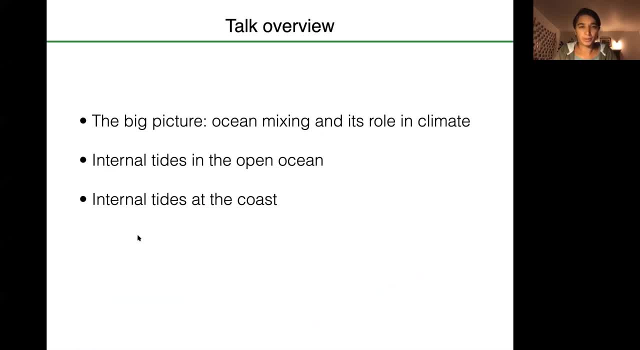 Oh, you can see it now? Yep, Okay, All right, Good, So the overview. very quickly. I'm going to start big picture, explain the motivation, ocean mixing and its role in climate, And then I'll zoom in a little bit and talk about internal tides in the open ocean, which? 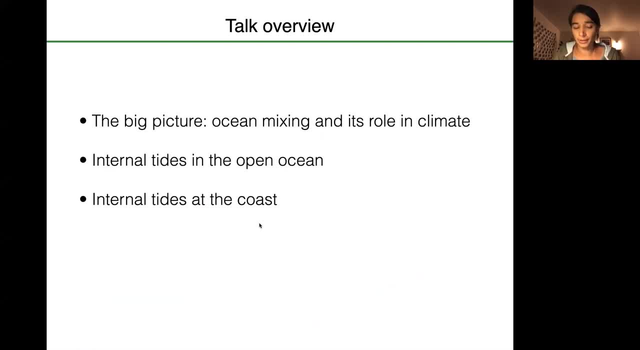 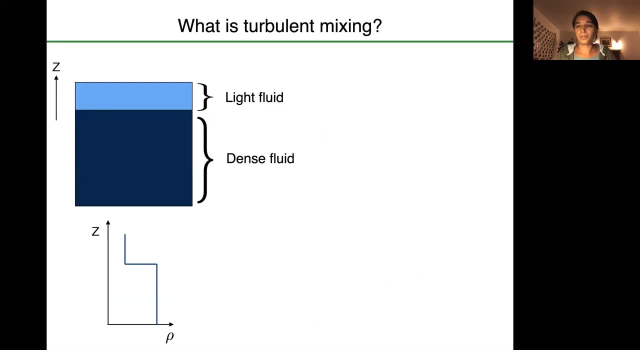 arguably, are better studied. And then I'm going to narrow down to my specific focus today, which is internal tides at the coast. So ocean mixing. you can see the next slide now, can't you? Okay, good, So let me just try and get everyone on the same page by explaining what I mean by turbulent mixing. 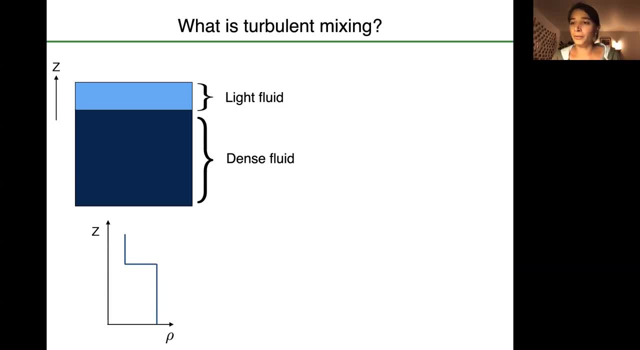 So imagine for a moment that the ocean only has two layers. It has a very light, warm layer that floats above a much deeper dense, a dense layer, a cold dense layer below, And so that's what I'm indicating here at the left, with this light. 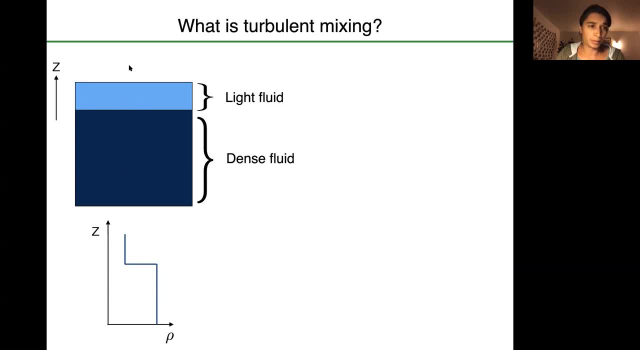 this light blue above and the dark blue below. If I was to pass a profiler from the top to the bottom, you would see something like what you can see in the bottom left corner here: less dense and then more dense, with a sharp interface in between. 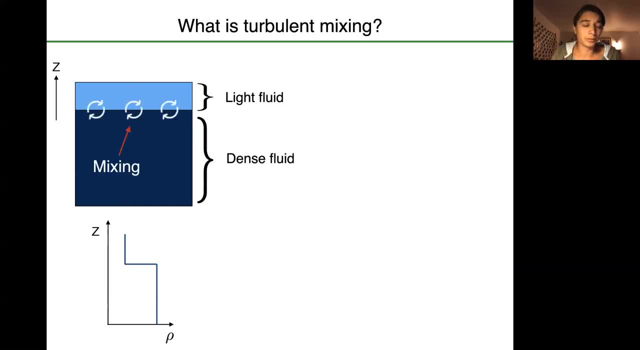 Now, let's say we add some mixing, So we add some turbulence to this. Well, what that mixing is going to do is it's going to generate, it's going to create an intermediate density class. It's going to mix the upper and the lower layer. 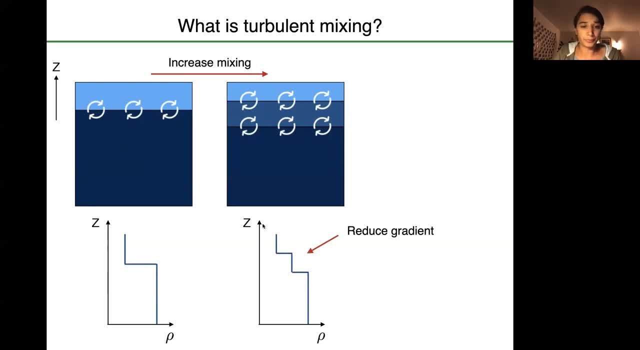 It's going to create an intermediate density, And so now, if I pass my profiler through here, you'll see a slightly reduced gradient. And so if I keep on doing this, I keep on mixing, I keep on creating these intermediate layers and I'm reducing the gradient. 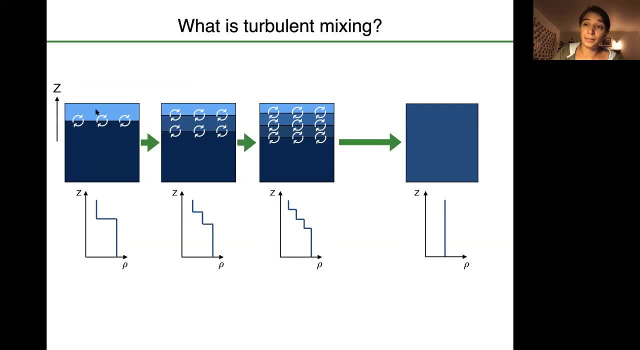 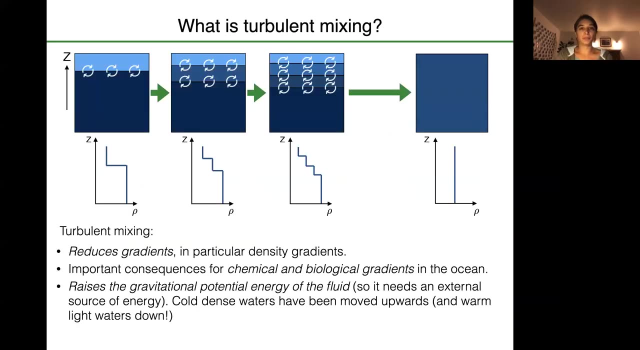 between the light fluid at the surface and the dense fluid at the bottom, And if I let this thing run to the end, then what I'll do is homogenize the entire fluid. So there is no density gradient whatsoever, And so what turbulent mixing has done here is reduced. 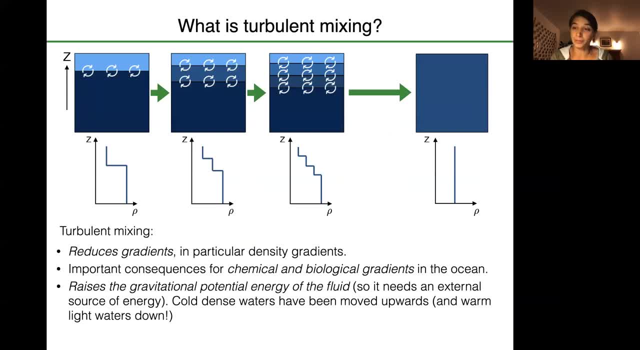 gradients, And as a physical oceanographer, I'm particularly interested in density gradients because they're very dynamically important. Obviously, this also has consequences for chemical and biological gradients in the ocean. From a physics point of view, what mixing has done is it's raised the potential energy of the fluid, And so you can see this if you consider the 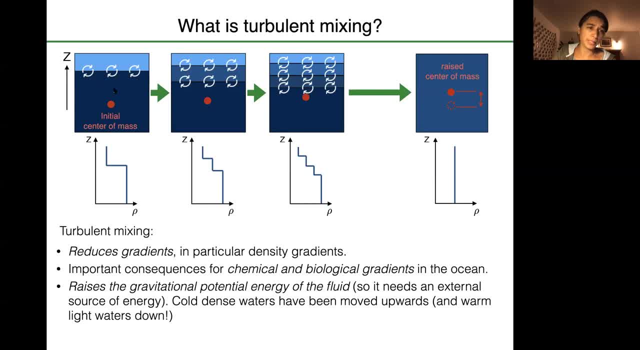 position of the center of mass of the fluid. In the stratified fluid, the center of mass is ever so slightly below the center of the depth, And as we mix the fluid, the center of mass is raised until it's in the center of the fluid, And so the potential energy of the final system is. 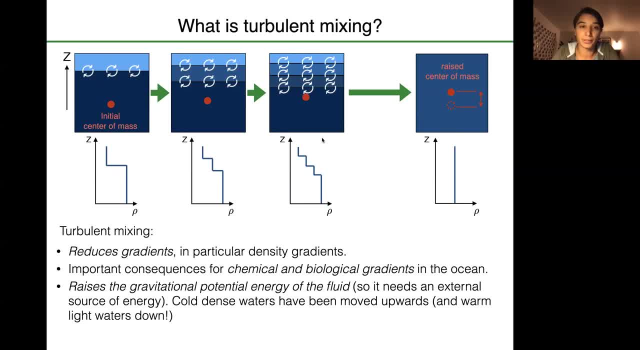 more than it was in its initial stratified state. So conservation of energy requires that mixing requires a source of energy. It's required a source of mechanical energy, And in the ocean that tends to come from the winds and the tides. So why do we care about mixing? Well, it's obviously 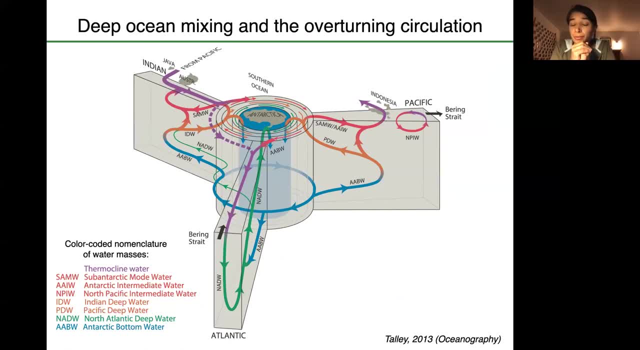 it's a fundamental ocean process. It happens. The ocean has an extremely large Reynolds number: 10 to the 8. So it is turbulent And mixing is occurring everywhere, on relatively small scales, scales of tens of meters, I would say- But it is ubiquitous. 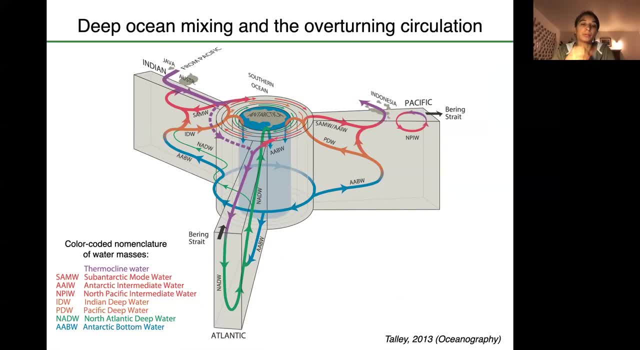 And, as a result, it has an influence on climate, And so what I'm going to show here is how is how turbulent mixing plays a role in global climate, using the schematic from Lynn Talley 2013.. So what she's done here, she's split the ocean into three ocean basins. So these are the 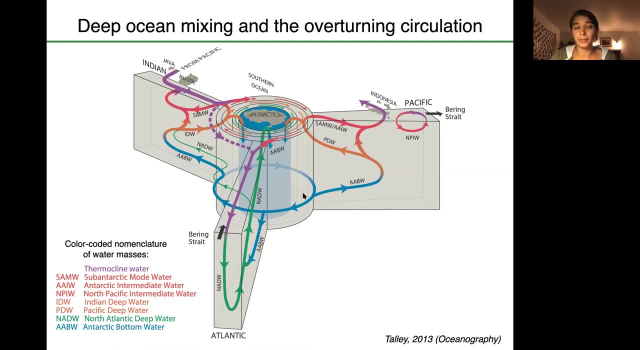 boxes here: the Indian, the Atlantic and the Stellar and the Pacific, and then the Southern Ocean, with the Antarctic circumpolar current going around Antarctica, And then all of these arrows and colors. these indicate the flow of water between each of the ocean basins And you don't need to worry too much about the water masses that are. 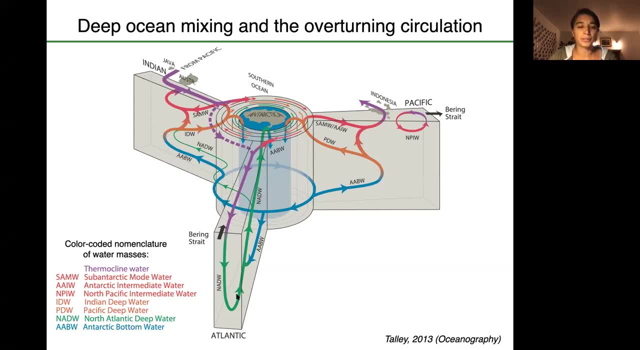 labeled Atlantic bottom water, etc. Just that water does pass through each of the ocean basins in this large scale, overturning circulation, And so, conceptually, I like to think of this. I'm a simple kind of person, so I like to think of this in three parts, And so the first part. 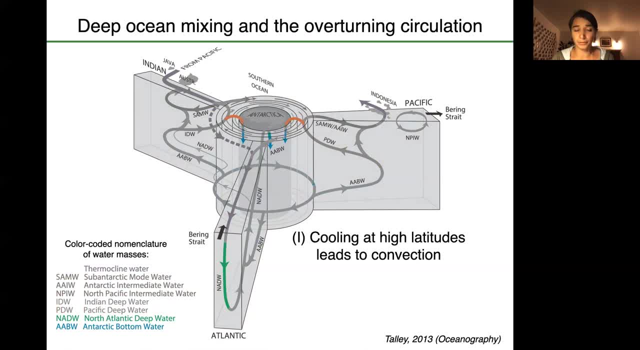 is the formation of deep waters at high latitudes, And so this occurs due to cooling in the winter. high latitudes when the ocean loses a lot of heat at its surface and it forms dense fluid, the densest fluid, And so this is the formation of deep waters at high latitudes, And so this 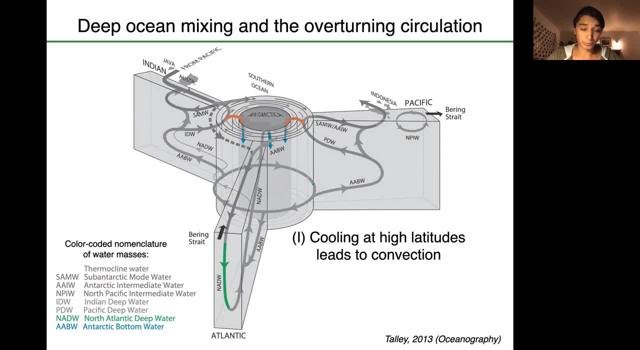 is the formation of deep waters at high latitudes, when the ocean loses a lot of heat at its surface and it forms dense fluid in the ocean that sinks to the bottom And it forms the densest water masses, the Atlantic bottom water and the North Atlantic deep water. Deep water formation only. 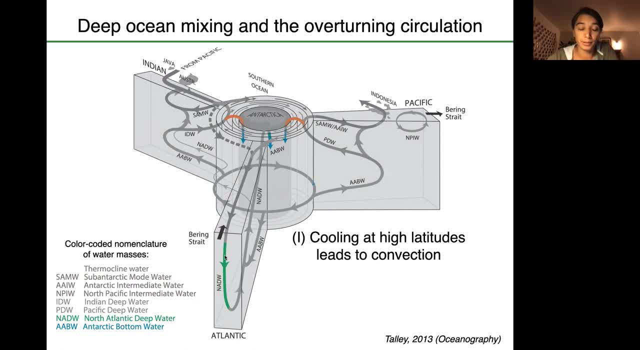 occurs in the Southern Ocean and in the North Atlantic. Now, once that deep water has formed, there are two ways by which that water can be returned to the surface. So intermediate depth waters can be drawn back up to the surface without a change in their internal energy. 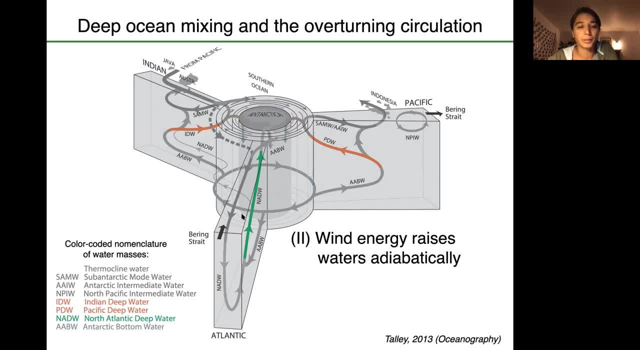 Three of the ways that deep water can be drawn back up to the surface can be drawn back up to the surface. can be drawn back up to the surface through the action of wind stress in the Southern Ocean, And this happens because these isopitinols outcrop in the Southern Ocean And so they can. 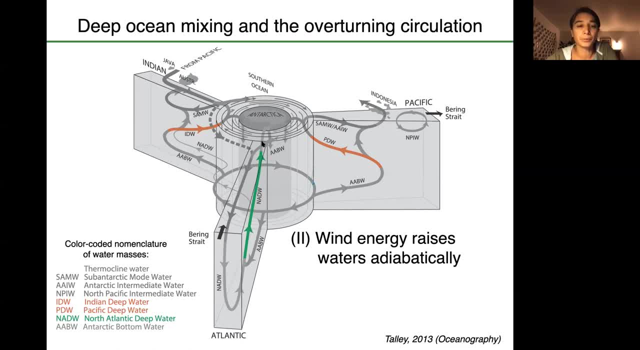 essentially slide up an isopitinol simply through the action of wind stress, without having to change their density, And so that accounts for the shallow cell of the overturning circulation, And that's essentially determined by wind stress. the rate at which that overturning occurs is. 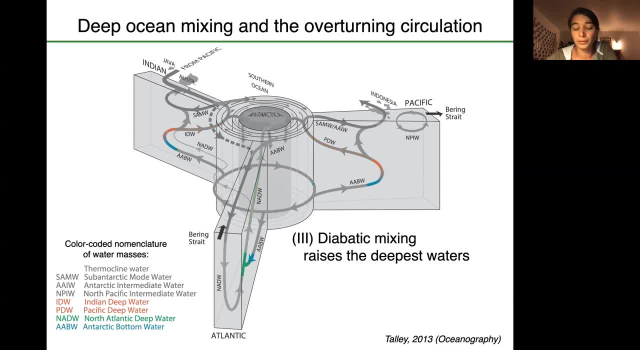 determined by wind stress. However, there are other ways that deep water can be drawn back up to the surface to precision, And they do appear quite 메�rior. However, the deepest waltzes really rely on turbulent mixing to return to the surface. There are no shared isopitinols with that deepest water. 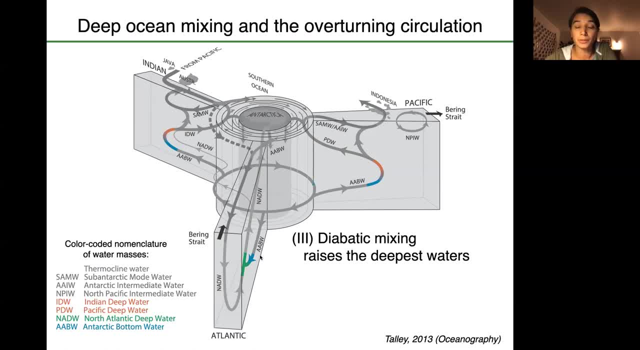 at the surface And the only mechanism by which they can return to the surface is by the ед勿m Rowling os by dragadan d. so this has implications when we come to, when we come to try and project how ocean circulation will change in the future using numerical models. The 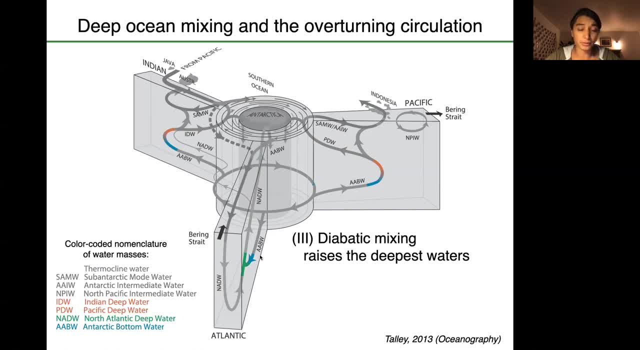 is that turbulence occurs at small scales, so, as I said, tens of meters, and when we model climate, we tend to do it at very large scales because we want to run simulations for hundreds of years and we want to couple both atmosphere and ocean together. So I believe that the IPCC class of 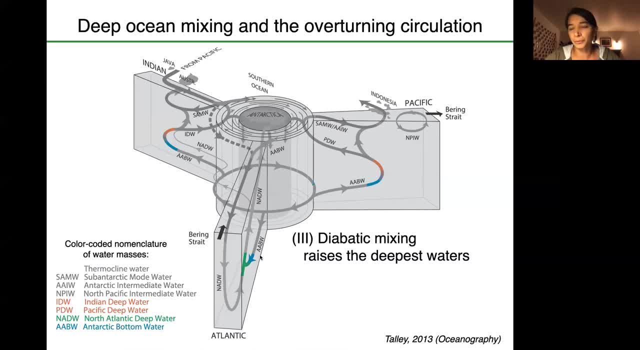 global climate models are at scales of around about one degree, so of order 100 kilometers, and so it's impossible to represent, or it's impossible to model turbulent processes in these models and it kind of will be for the foreseeable future. So it's necessary to represent. 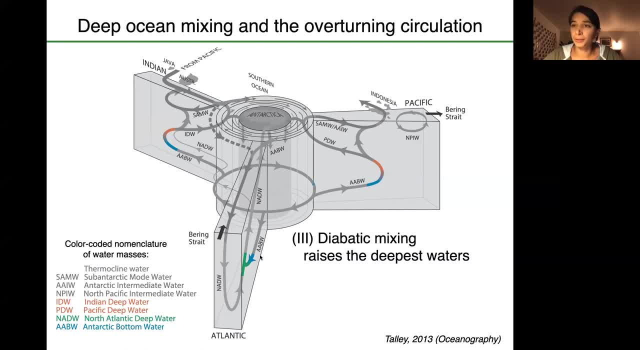 the impact of turbulent mixing in these models, and so this kind of leads to this cottage industry of trying to develop parameterizations, physically based parameterizations, for when and where turbulence mixing occurs. turbulent mixing occurs in the ocean, and so that that's really. 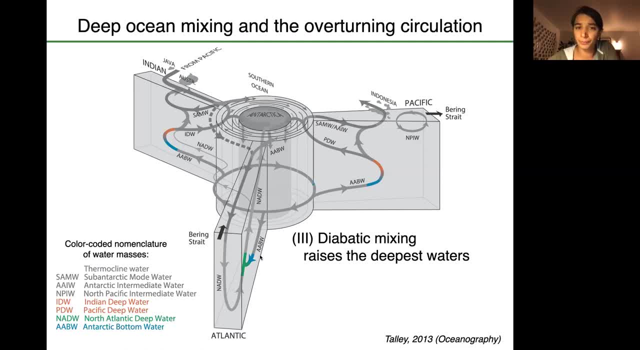 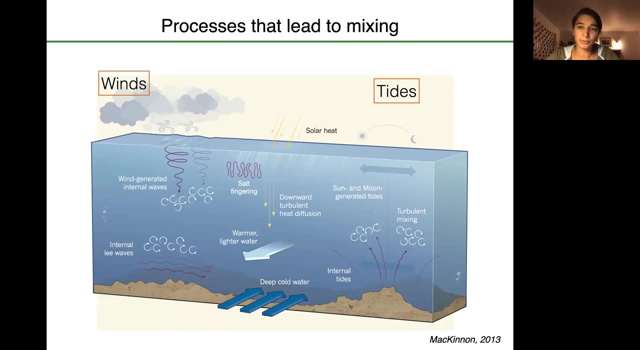 really important, The main motivation, for me at least, for trying to understand when and where mixing is happening in the ocean. Now, there are a number of different processes that lead to mixing, but essentially the source of energy for mixing comes from either the winds or the tides, so the 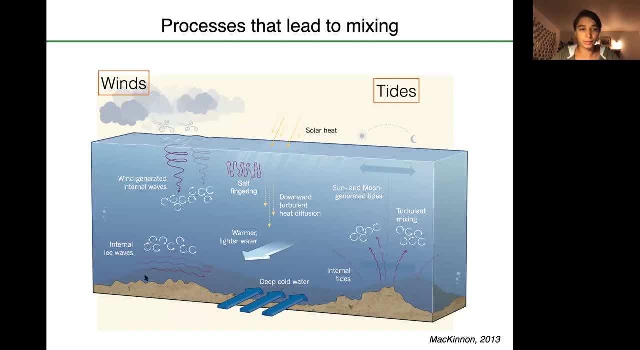 schematic comes from an article by McKinnon in 2013.. On the left side of the schematic, you can see the wind associated processes. so the winds blow over the surface of the ocean and, for the purposes of mixing, they do two things. They generate wind-generated internal waves, which 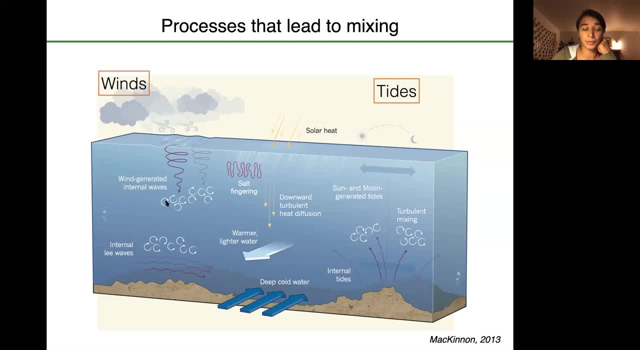 can propagate down into the interior of the ocean, where they can then break and mix and the winds also set in motion the general circulation, the low frequency flows and the deep currents that can interact with topography and generate lee waves. Those lee waves can lead to turbulence and 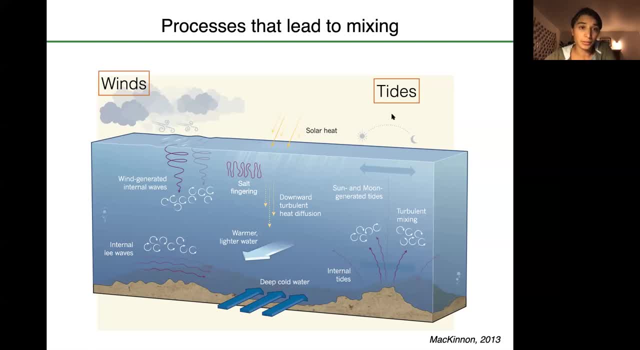 and mixing. close to the bottom of the ocean, The tides also can lead to mixing, and the tides- the tides- dissipate around about one terawatt of energy in the ocean, which is comparable to the work done by the winds on the ocean. so each of these, each of these processes is equally important. 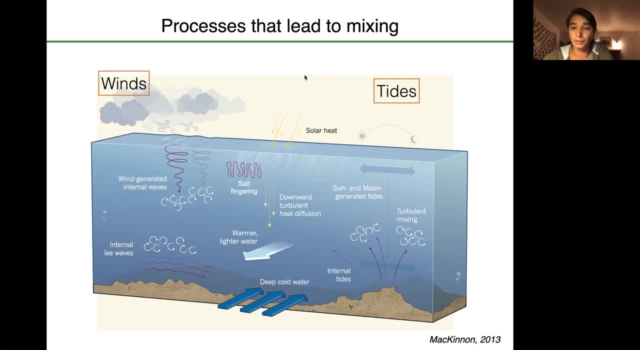 in dissipating energy in the ocean and potentially leading to mixing. So the tides- which is the focus, the focus of what I'm going to talk about here- the tides generate internal tides, so these are internal waves at tidal frequencies that can, that can propagate energy elsewhere through the ocean. 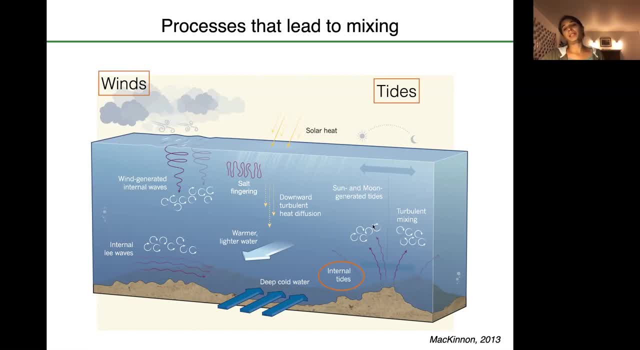 and they can lead to mixing, And so the energy pathway that that I think is is understood. for the tides is that the surface tide, the tide that we're most familiar with, that we see when we go to the beach, and we see the surface of the ocean advance and recede. 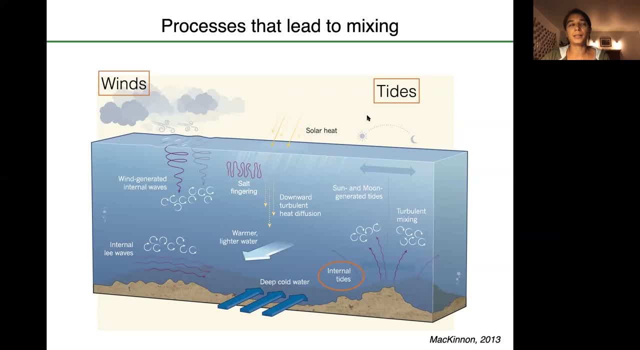 twice a day, or once a day, depending on where you are. that tide, the energy for that tide, the surface tide of the barotropic tide, comes from the energy in the astronomical configuration of the earth, moon and sun. That energy is then transferred into internal motions. 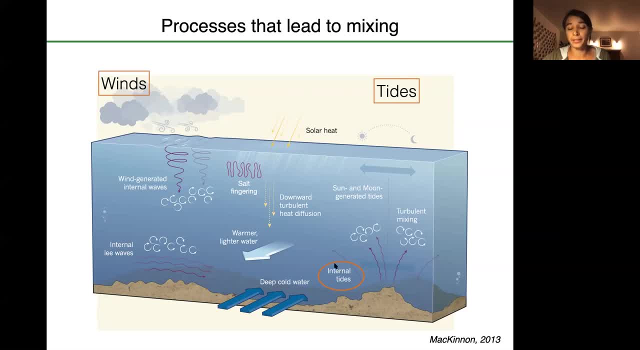 in the internal tides, and the internal tides then transfer that energy throughout the ocean basin before they break out. And that's the way that the energy of the ocean can mix and lead to dissipation, ultimately the dissipation to heat of that energy. And so the first step in this pathway is: 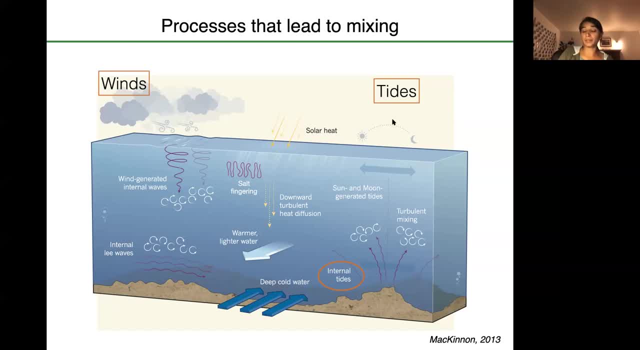 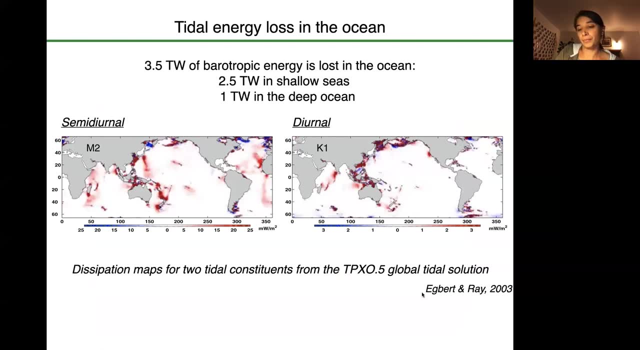 understanding where the barotropic tide is losing energy, and we have maps of this. So these maps were created by Egbert and Ray in 2003. and what they did? they've used altometric measurements constrained to a simple model to examine where the barotropic tide is losing. 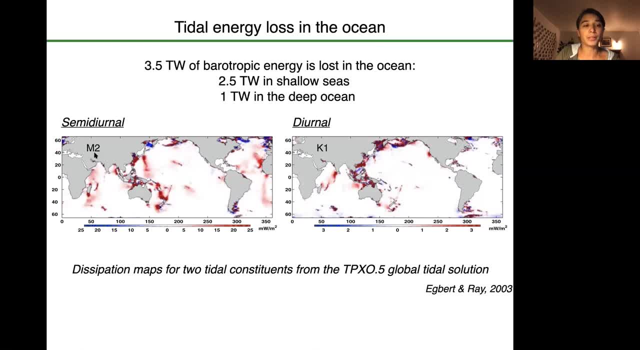 energy in the ocean for two major tidal constituents: the semi-dianal M2 and the diurnal K1. And where you're seeing red, this is where the barotropic tide is losing energy. Overall, they found that the barotropic tide loses energy at a rate of 3.5 terawatts in the ocean. 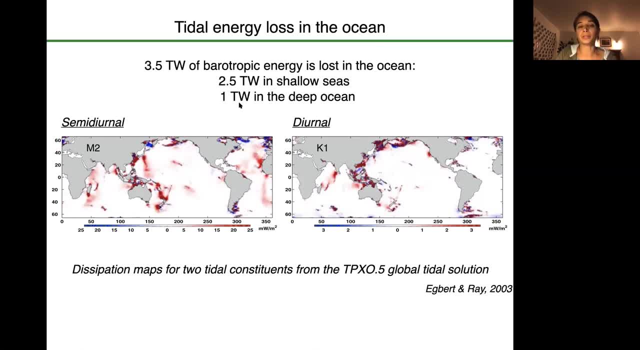 4.5 terawatts is dissipated in the shallow seas and 1 terawatt is dissipated in the deep ocean, And so, just looking for a moment at only the semi-dianal constituent, you can see that there's. 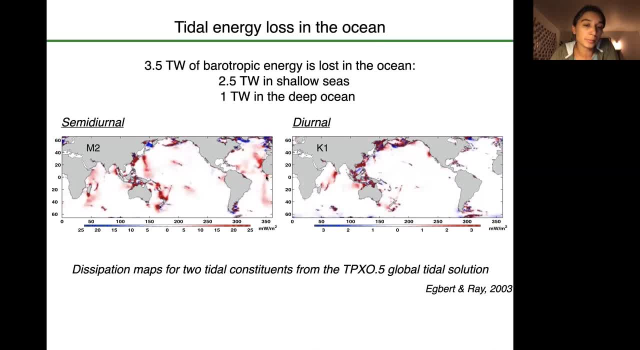 a significant loss of energy over these features that turned out to be correlated with topography in the deep ocean. So this is Hawaii, this is the Mariana Ridge, this is the Mid-Atlantic Ridge here, And what's happening here is that the barotropic tide is. 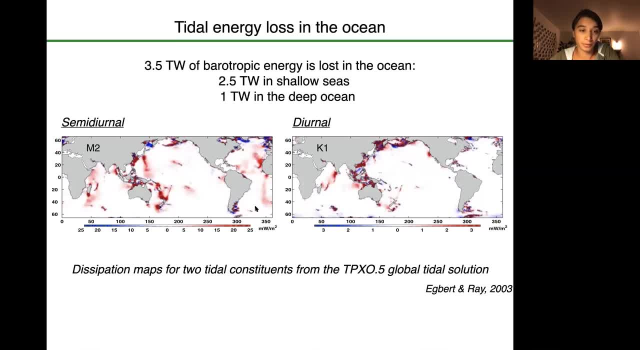 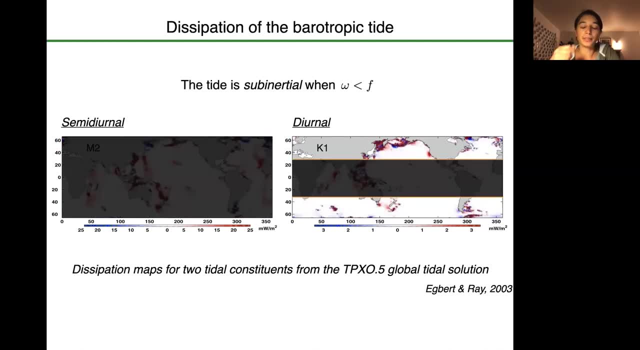 conversing its energy into internal tides that can transfer the energy away. Now it's a little bit more complicated than this, because actually the exact nature of the internal response of the ocean to that barotropic forcing depends on the frequency of the forcing. 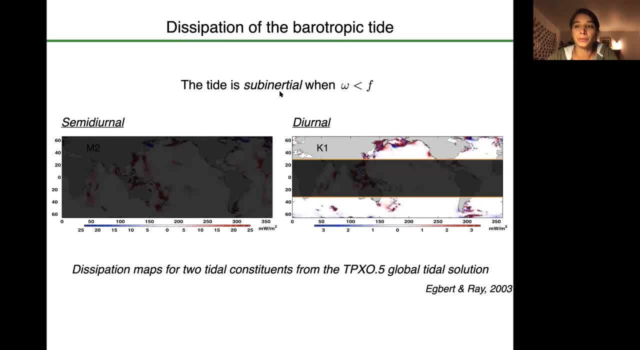 And so I'm going to talk about the tide being subinertial or superinertial. When the tide is subinertial, it has a relatively low frequency compared to the local Coriolis frequency. So these are low frequency tides. So the diurnal tide, which is once per day, 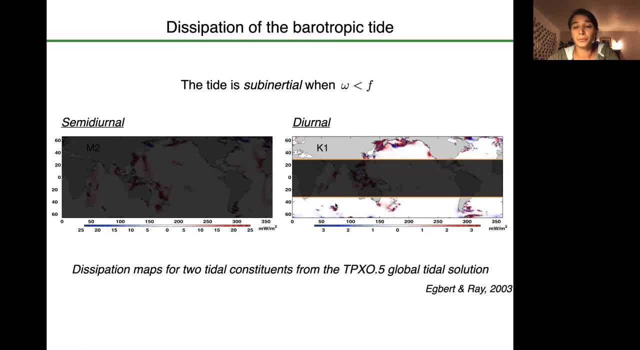 is subinertial everywhere- polewards of 30 degrees. The semi-dianal tide is only subinertial polewards of about 74 degrees, And the response of the ocean to subinertial forcing is very different compared to when it's. 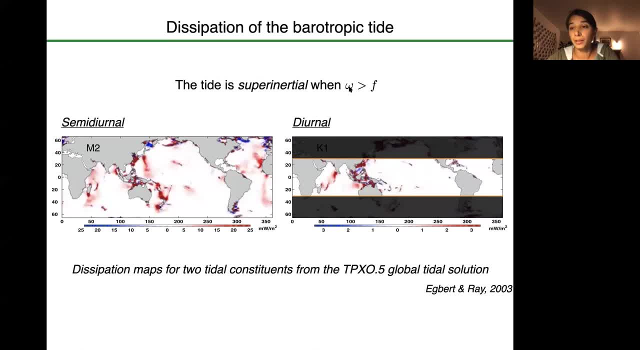 superinertial, And so when it's superinertial, these are relatively high frequency tides. The semi-dianal tide is superinertial over much of the ocean basin And the response, the dip, the dissipation or sorry, I should say, the loss of energy from the barotropic tide. 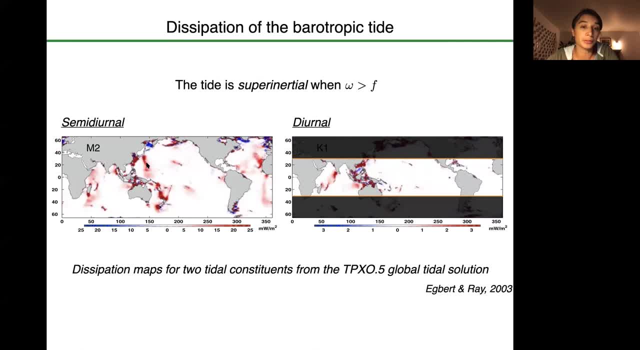 is mediated by the physics that arises from superinertial interactions of a stratified fluid with topography. And so, to understand what that looks like, I'm going to show you the output of a numerical model, And so what this model has done. this was run by Simmons et al in 2004,. 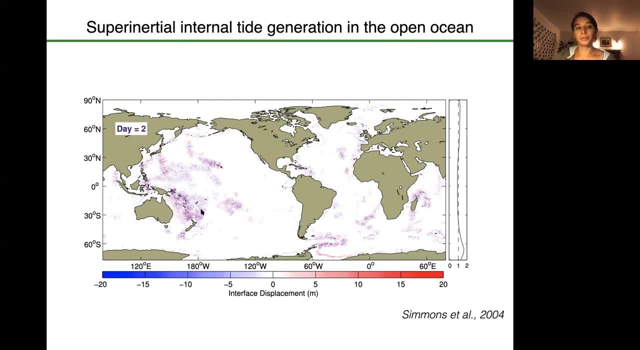 they took a global, global model and they imposed uniform stratification everywhere. So this is stratified fluid and they applied a tidal forcing. And then they looked at the interior response of the model, And so what you're seeing here in red and blue is the interface displacement. 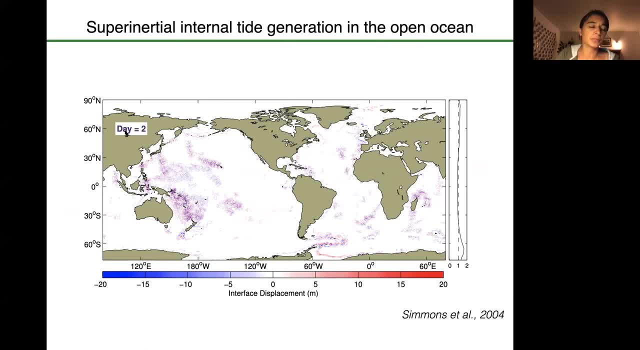 I think at around about 100 meters or so, after two days of the simulation, And what you can see around these regions that came up in the maps of of barotropic tidal loss, you can, you can see the generation of these internal tides. 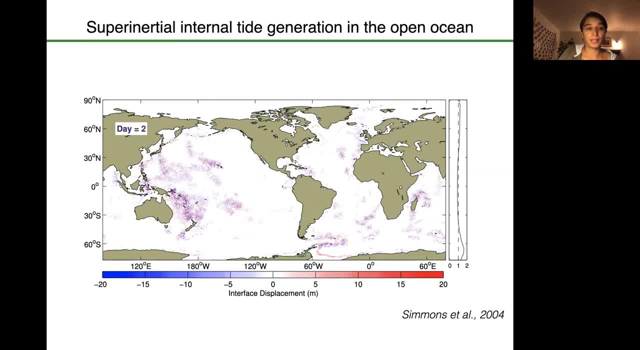 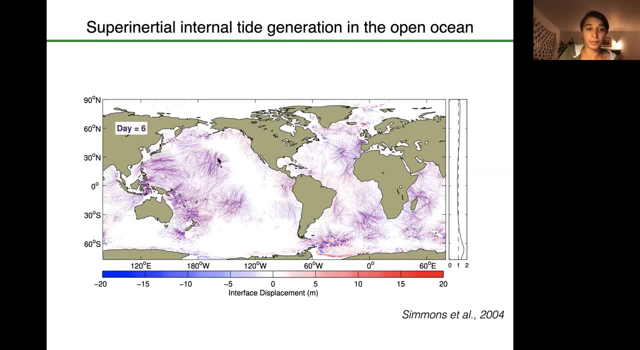 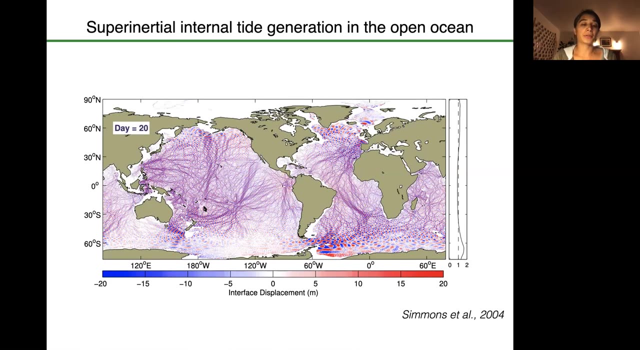 these waves radiating away with small scales. After six days, these, these tides, have really radiated long distances, expand, transferring energy from their generation sites throughout the ocean basins And after 20 days, you can see that in this very idealized global simulation, the entire 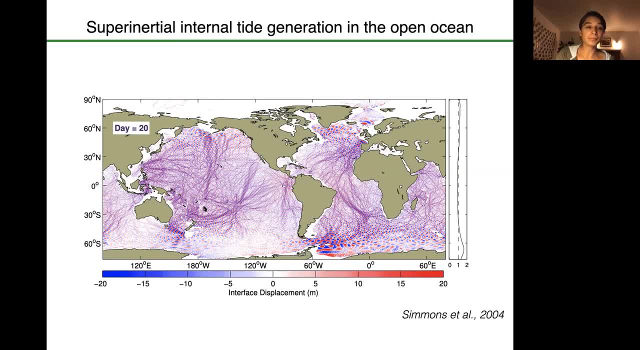 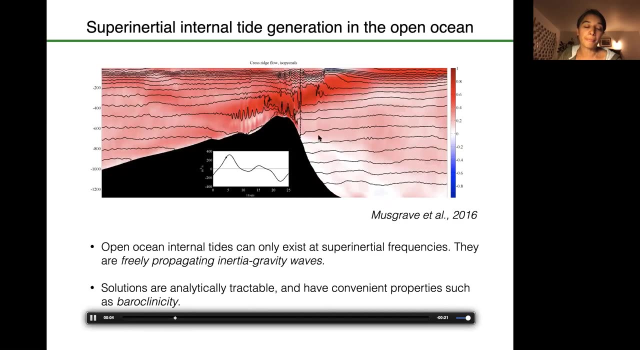 ocean is full of internal tide And they also see the geyser system, which is having a very large thought process, which actually takes a lot of energy to get a sense of what this looks like under the water. for for those that don't, 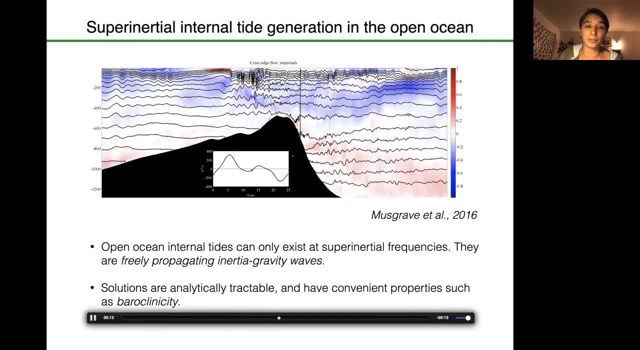 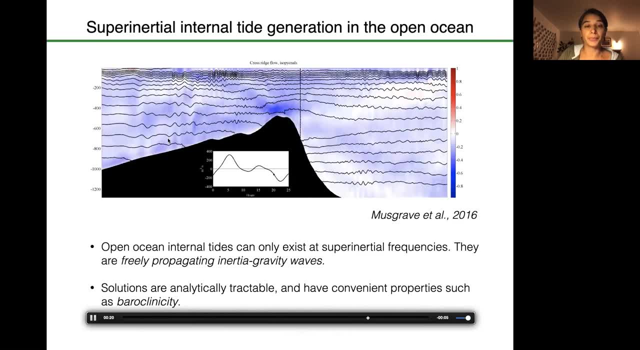 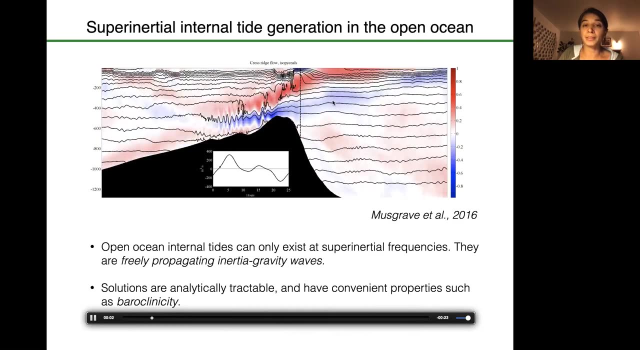 don't necessarily research this and see it every day. This is another simulation. this is one that I ran, And so this is now looking at a cross section, cross ridge tidal flows, and so what you're looking at here, the black lines are isopitinols and the colors are the currents. they're actually the. 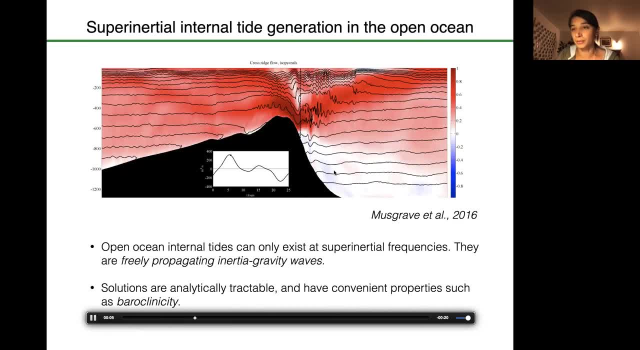 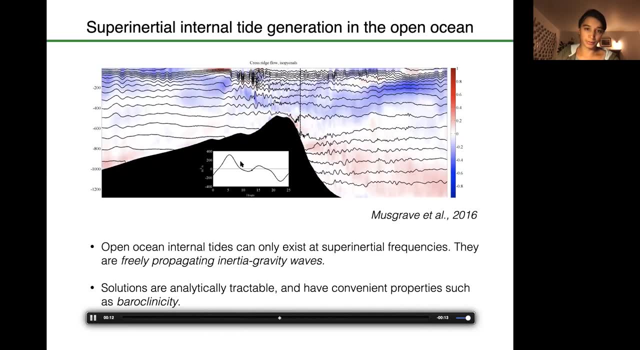 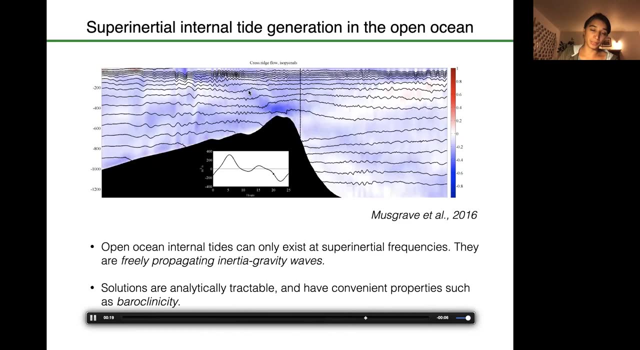 baroclinic currents, so I've subtracted the depth mean to isolate the internal tide response and there are a couple of things to see here. the first is most of the energy that, most of the energy that is being extracted from the tide that I'm- the barotropic tide here- is being conversed into an internal tide. 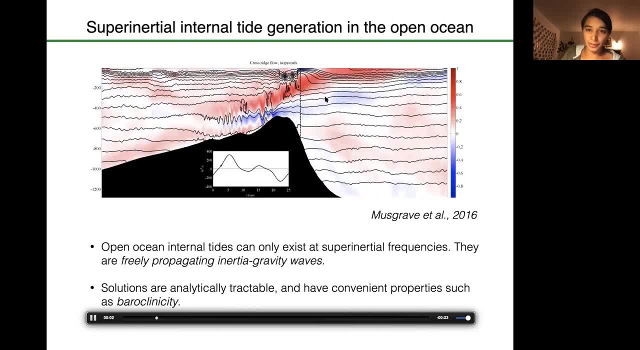 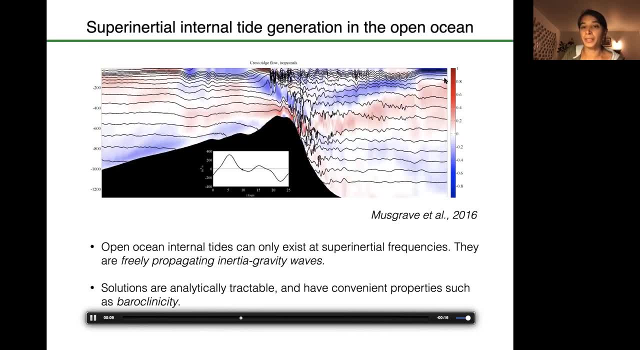 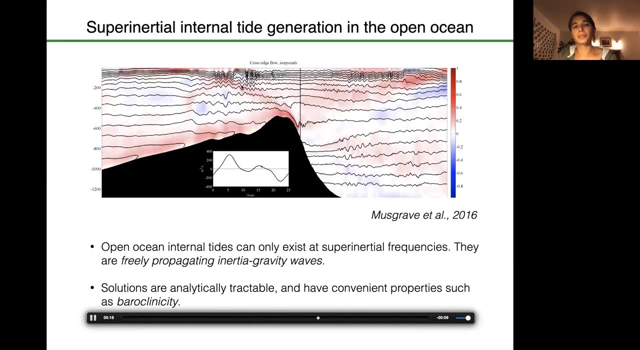 that propagates away from the ridge, and so you can see the formation. these are internal tide beams, internal waves. the phase is propagating down. the group energy is radiating outwards, so it's radiating outwards to the right and to the left of the screen. there's also some local dissipation here, so you can see. 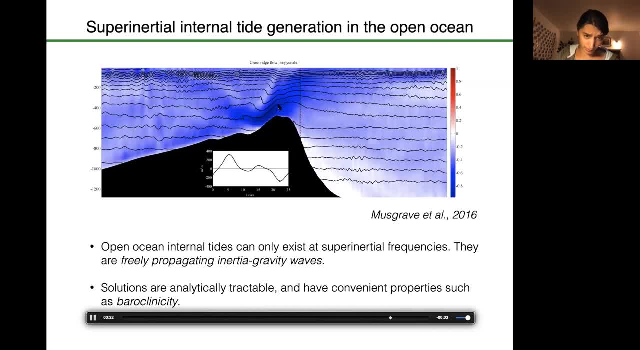 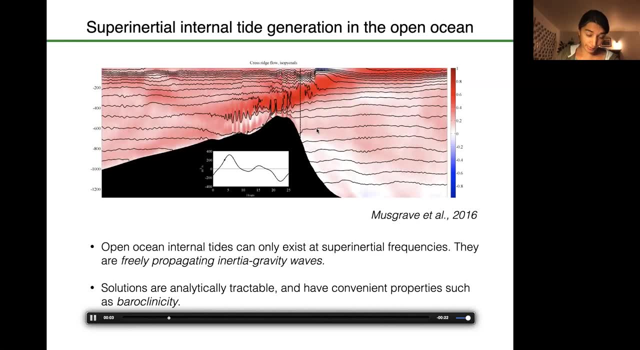 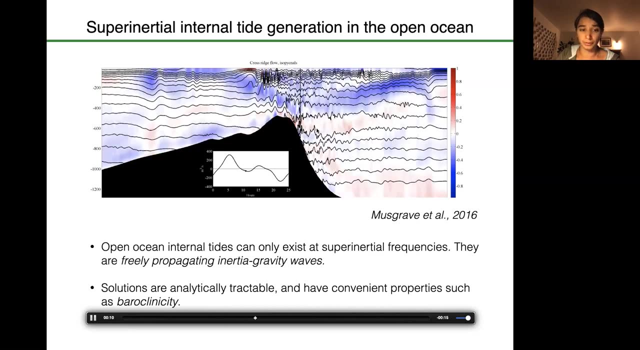 how these internal waves can break in this particular location. things become very non-linear, the waves become the isopitinol displacements, become very steep and they overturn much like, much like breakers at the beach. when you see, when you see waves shoaling at the beach. now the nice thing about super inertial internal. 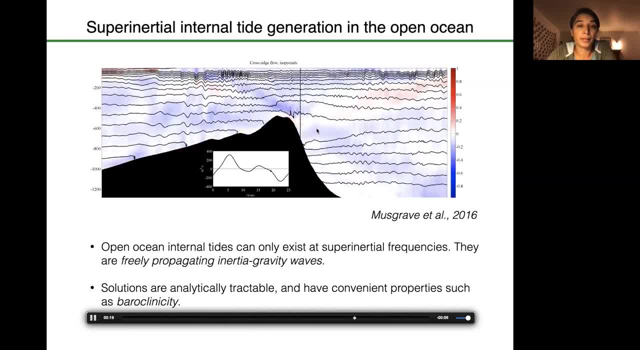 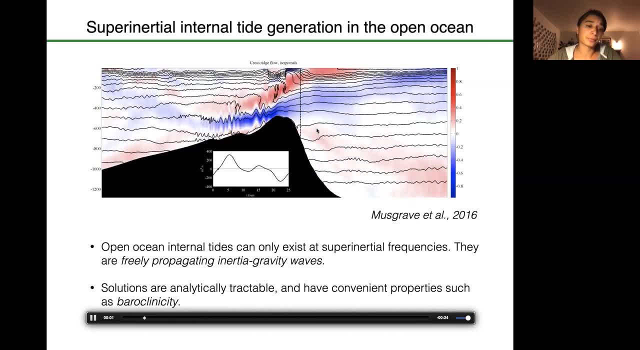 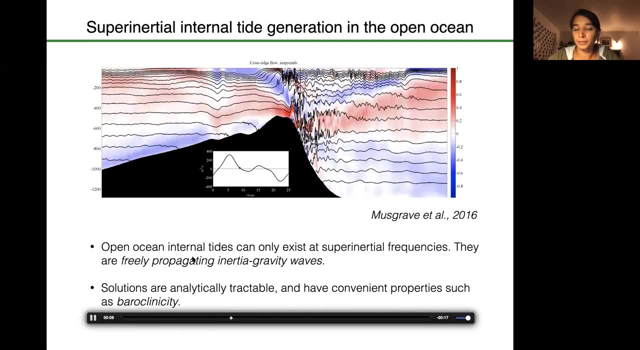 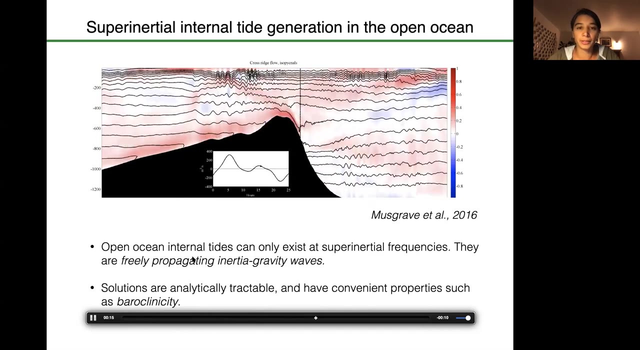 tides is that? well, they. they are of a class of waves called inertia gravity waves, freely propagated propagating inertia gravity waves, and they have some very nice properties that make them very easy to work with, that analytically quite tractable, and I'm going to go through this on the next slide with a little bit of mathematics. 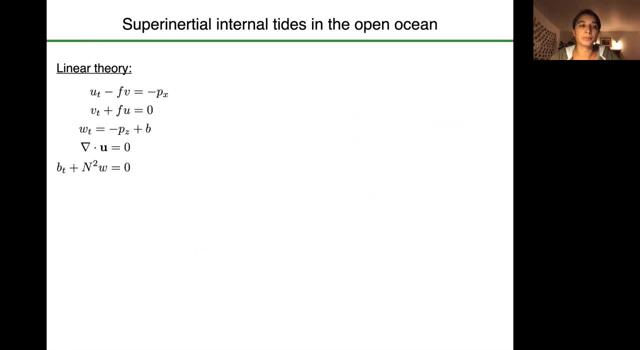 it's just one slide, but I do think it's helpful to compare the response when we have subinertial tides over coasts, so that you can kind of see how these two things are different side-by-side. and so the the theory is is pretty straightforward. we start with a linearized set of equations, the 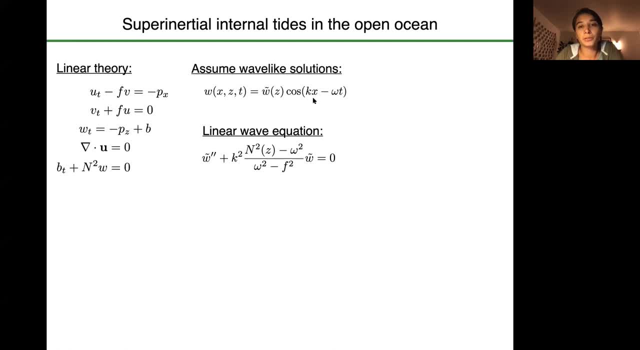 Navier-Stokes equations and we assume that the solutions are wave-like, they're periodic, in X they have a frequency that is equal to the tide, the forcing frequency, and they have some unknown structure in Z, and we can combine the governing equations to form a single wave equation, a field. 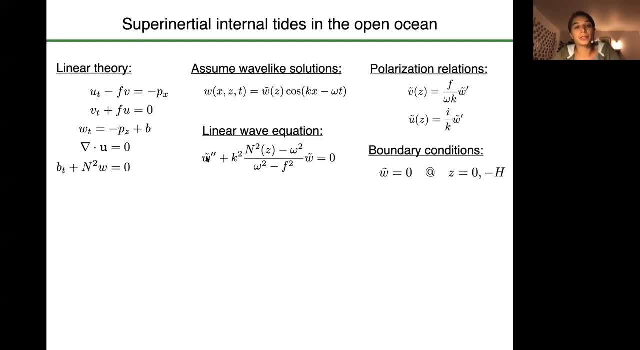 equation and then essentially. so. this is for the vertical velocity component. W say quite reasonably, over flat bathymetry the vertical velocity should be zero at the bottom of the ocean and zero at the top of the ocean. And so if we impose that as boundary, 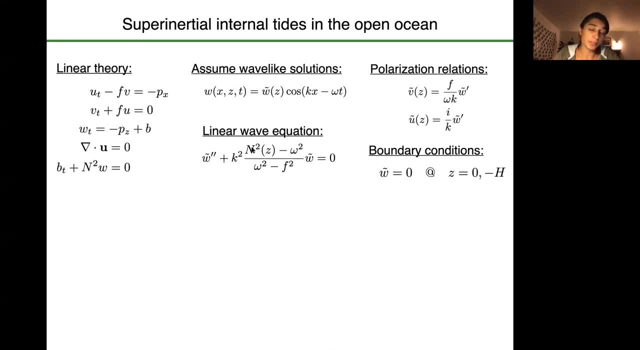 conditions. hopefully you can see that if we assume that n squared, the stratification is constant with depth, solutions to this are simply signs, sinusoids. they're just signs, And so when we allow n squared to be a function of depth, then we can solve this. 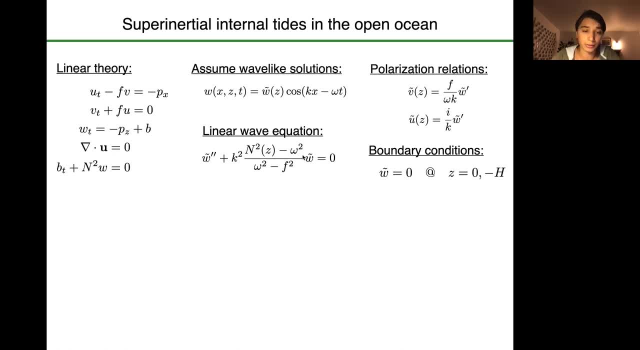 equation numerically, but it still is just an eigenmode equation, And so here's an example of a solution here. So I've taken a stratification profile from just off the Oregon shelf and I've solved this system of equations- this or this equation- with this boundary condition. 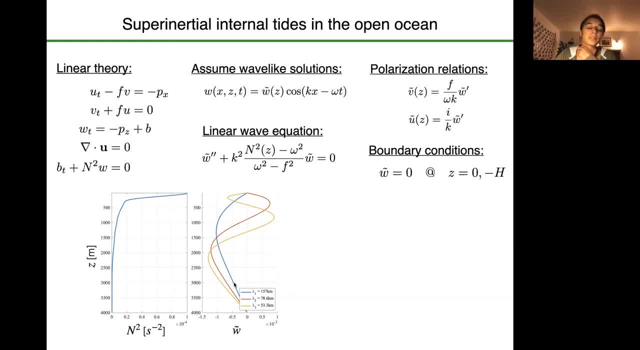 and this is what the modes look like. So the takeaway point here is that the modes are only innovative, So the mode one is just the vertical over a flat bottom, and they're increasingly complex for higher modes. So mode one is just the first sinusoid and mode two has an extra. 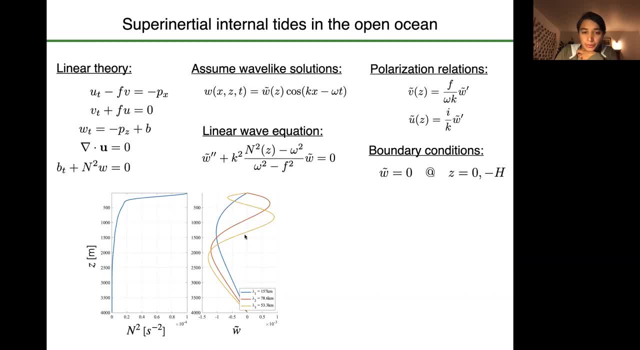 crossover. Mode three has two crossing points. at zero, There's a dispersion relation. as you might anticipate for a wave problem, The dispersion relation relates in order for the fluid motion to satisfy this, This motion described by the modes, the wave number and the frequency have to be related. 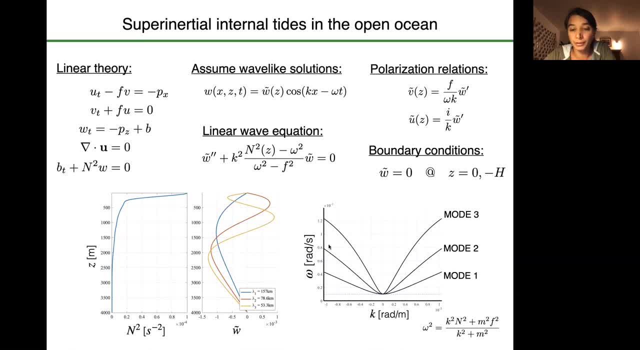 by this dispersion relation here, And this is what it looks like. I draw your attention to it because I'm going to show you more dispersion curves later and these will appear, But essentially the dispersion curve is kind of parabolic. You'll notice that these waves can't exist. 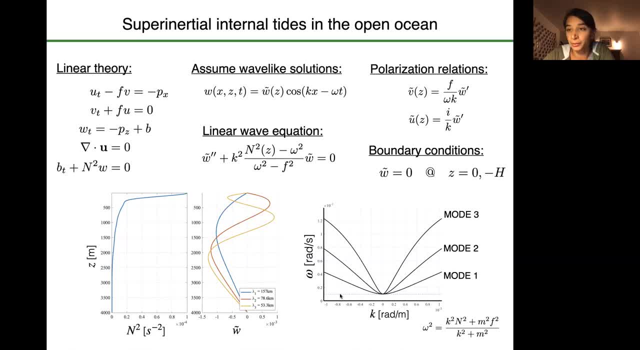 at subinertial frequencies. So this dashed line here: this is where omega is equal to f, So these waves are constrained to exist only at subinertial frequencies. So this dashed line here: this is where omega is equal to f, So these waves are constrained to exist. 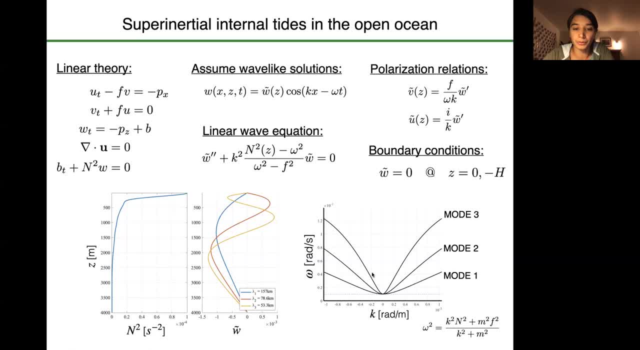 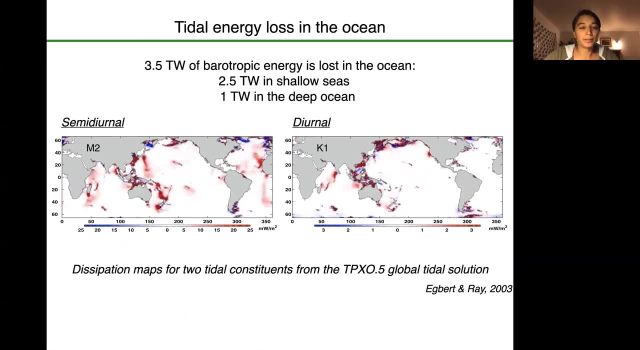 only at relatively high frequencies, for superinertial frequencies. So that accounts for that very simple theory. actually quite well describes the generation of internal tides where the tidal frequency is superinertial, So that's for the semi-dynamal constituent over much of the ocean and where the ocean floor is largely flat. So once you 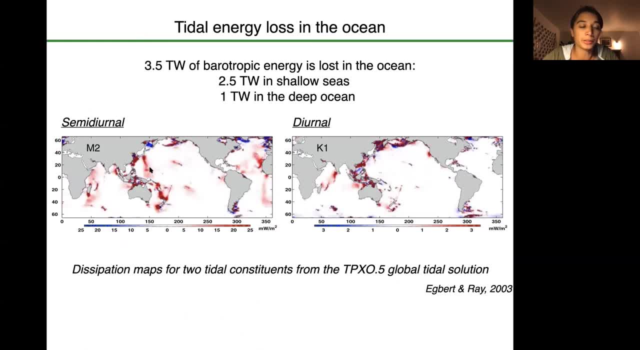 get away from Hawaii and once you get away from the ocean floor you're going to have from the Mariana Ridge. the ocean floor is largely flat and that theory well describes the propagation of these waves. However, in shallow seas, where we actually have most of the loss of energy from barotropic tide, the ocean floor is 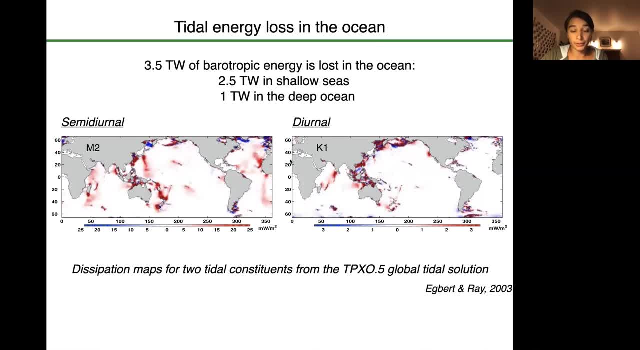 far from flat and furthermore, the diurnal tide, as I mentioned before, above 30 degrees north or below 30 degrees south, is sub inertial and so that that those wave dynamics don't apply there and so actually a different wave dynamics applies. And so to get at those, those wave dynamics, and we have to solve, 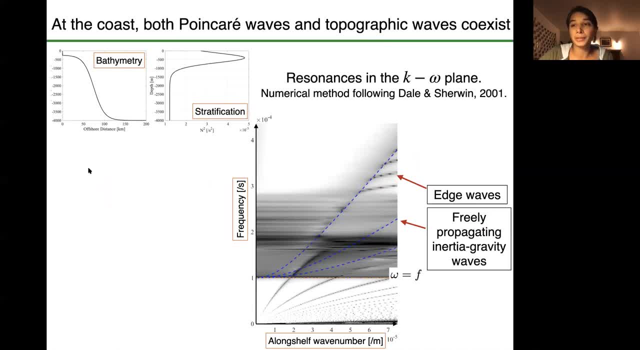 essentially it's the same equations as before, but now our boundary conditions are different, so we're going to apply a boundary condition of no flow along this sloping profile. so this profile represents the Shelfbridge, And in doing this we are no longer able to separate the 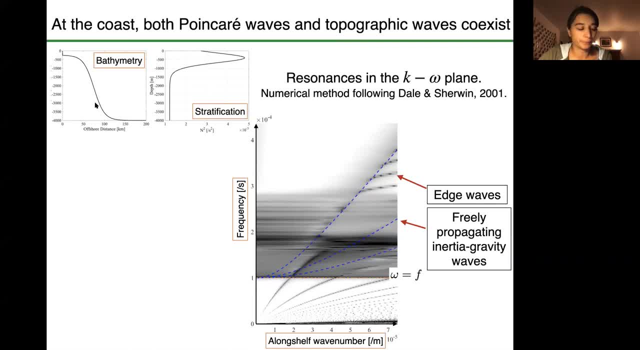 horizontal and the vertical components of the motion, so that the two dimensions become coupled. The methods for solving this- I mean it's just the linear problem- the computational method is slightly different, and the way that I'm presenting it here. this is a resonance scan and essentially what? 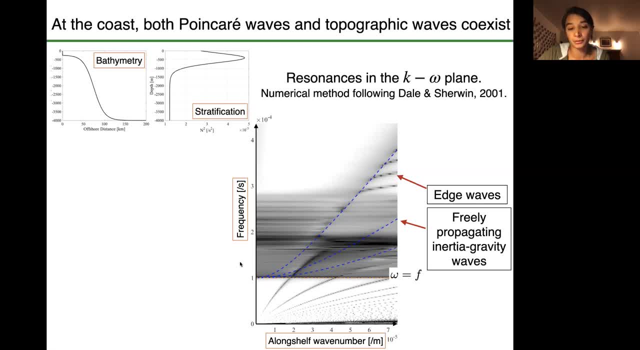 you're looking at here is a dispersion relation, so we have frequency and energy on this axis and wave number on this axis Where there are grey lines. so this is a pretty noisy plot for computational reasons. but where there are grey lines, this is where there are resonances in this domain, and so this is. 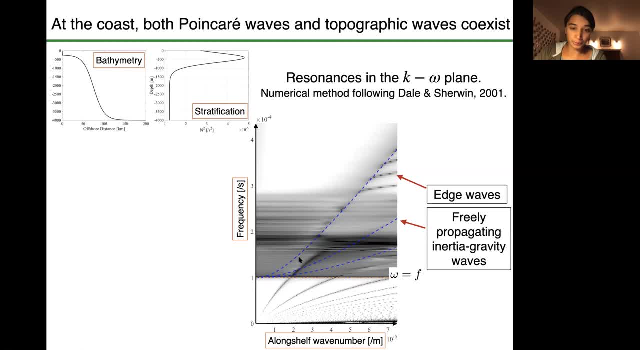 where the modes exist, And so the first modes that I want to draw your attention to, I've highlighted with these blue lines here. these are the freely propagating inertia gravity waves that I was talking about before. So these are super inertial frequencies and they do have a lot of pressure. They are able to. 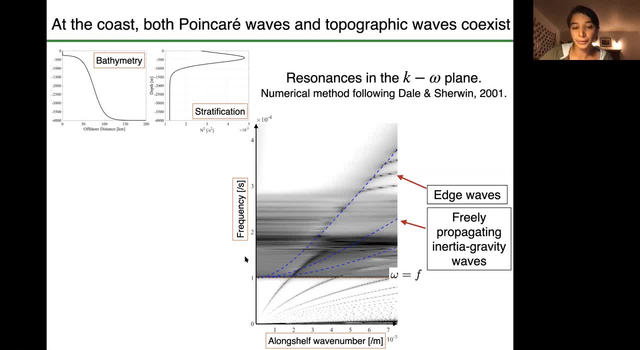 appear in this scan. However, there is an extra set of waves that I'm going to focus on now. These are the coastal trap waves, and they exist only because of the presence of the boundary. this bathymetric boundary supports them, And so what's interesting about these waves is that they 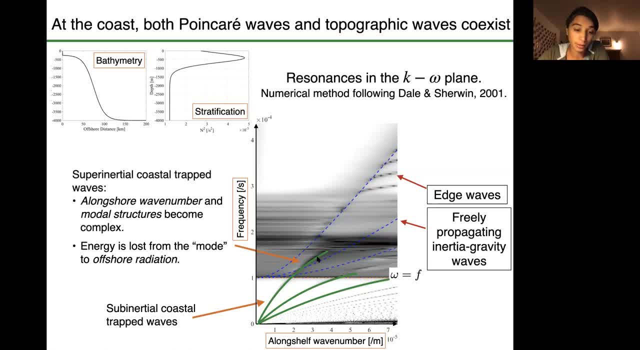 can exist at both subinertial and at superinertial frequencies. They only exist along coasts. When they are subinertial, they are completely trapped, so all of the energy is confined to the coast. However, when they become superinertial, they are able to exchange energy with the ocean. 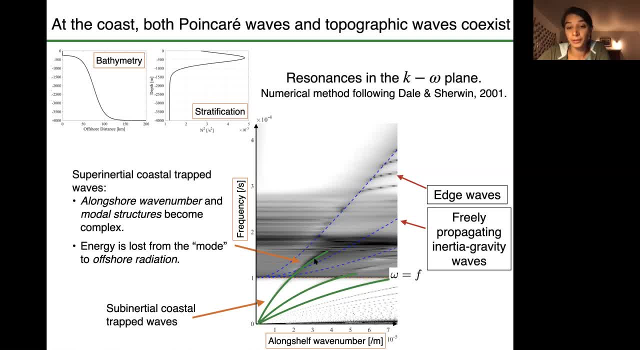 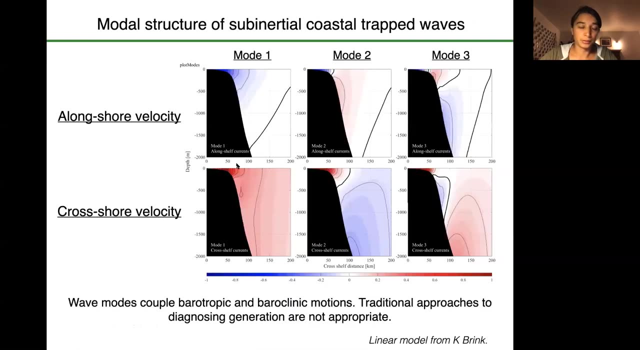 with the internal waves in the ocean's interior, and they're actually coupled to these freely propagating inertial gravity waves. So let me show you the structure of what these waves look like, at least in the subinertial case, just to give you a sense of what they are. 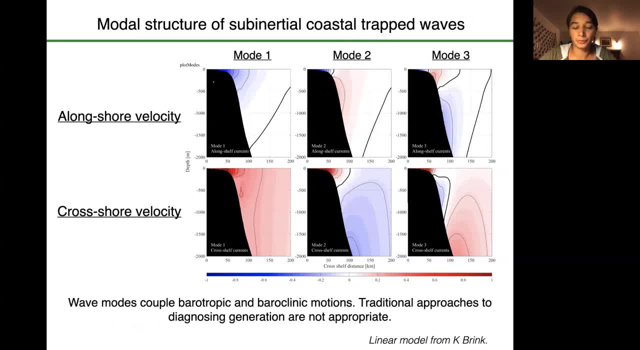 And so here's this bathymetry and I've solved that set of waves and I'm going to show you what they look like. So this is what the waves look like in the subinertial case. So this is what the waves look like. 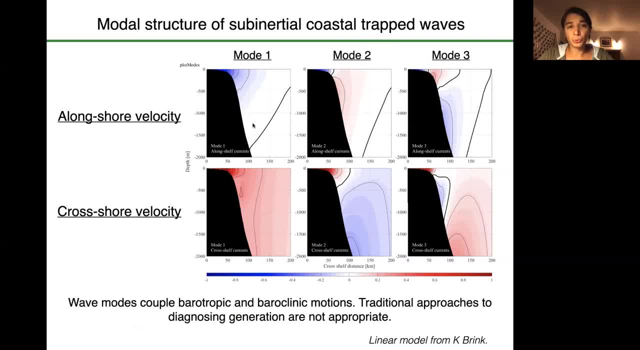 in the subinertial case. So this is what the waves look like in the subinertial case And these are what the modes look like. So mode one in the longshore velocity and the crossshore velocity. Mode two, slightly more complex. Mode three, even more complex, 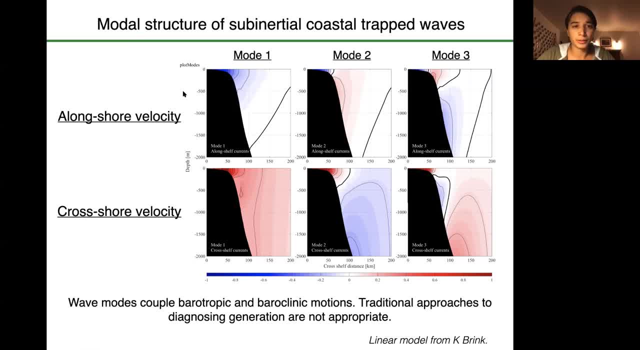 There's a couple of things that are important here. So the currents associated with these modes have a structure that is largely barotropic, so largely depth uniform on the shelf, But once you move over to the shelf break and over the slope they tend not to be barotropic. 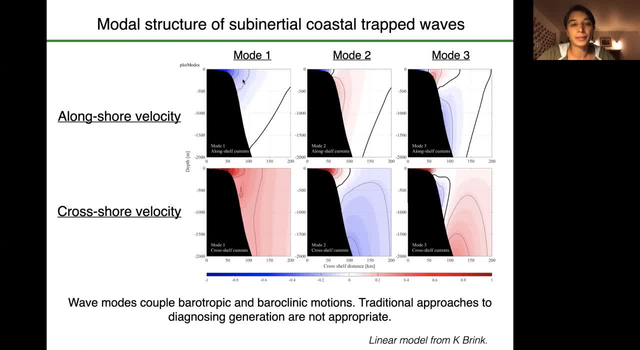 and this is the influence of stratification. They tend to acquire a baroclinic component and this is actually extremely inconvenient. So superinertial internal tides are baroclinic by definition over a flat bottom. That makes them very easy to work with with observations. 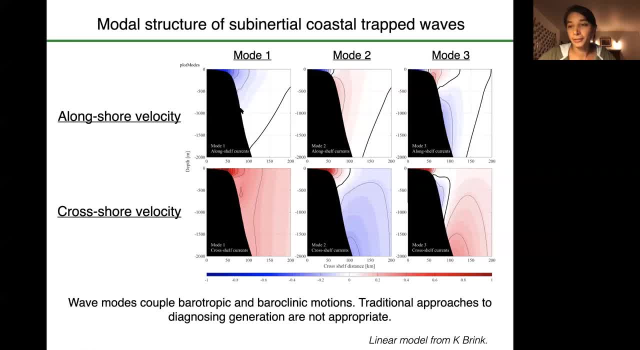 and in models All you need to do is subtract your depth mean, and then you're isolating your internal tides, And so there are whole frameworks for working with the energetics of these waves. that can't work over the coast because the dynamics couple barotropic and baroclinic motions. So this is 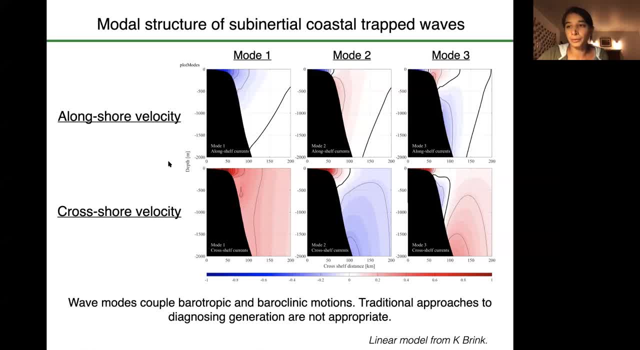 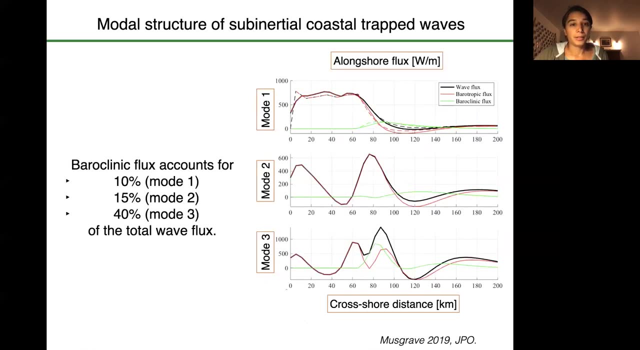 really just a practical issue. It's quite difficult to calculate energy transfers between modes and scattering of these modes explicitly in the same way that we do with superinertial tides in the open ocean. Just to kind of drive that point home, if we look at the 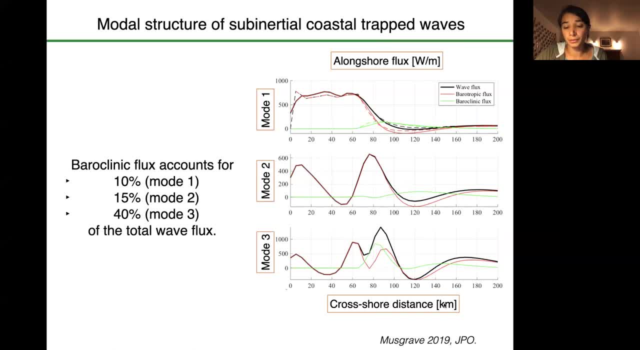 structure of the alongshore flux in these waves. so this is the cross-shore distance here, and what I've done is I've calculated the alongshore flux from these modes- mode one, mode two and mode three. The alongshore flux also has a fairly complicated structure, So 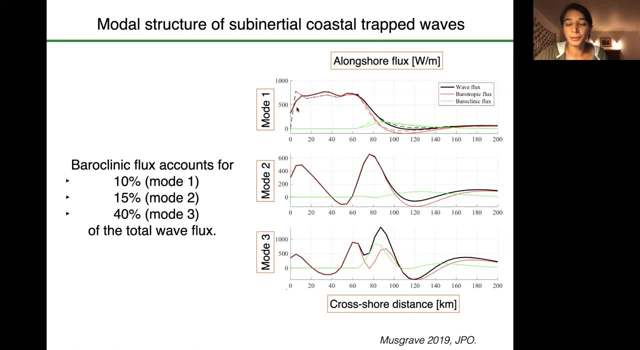 if you go out and measure at one location, you won't really capture what the total flux is. The total flux is really the integral of the cross-shore direction And, as I mentioned before, the flux and the motion tends to be largely barotropic. 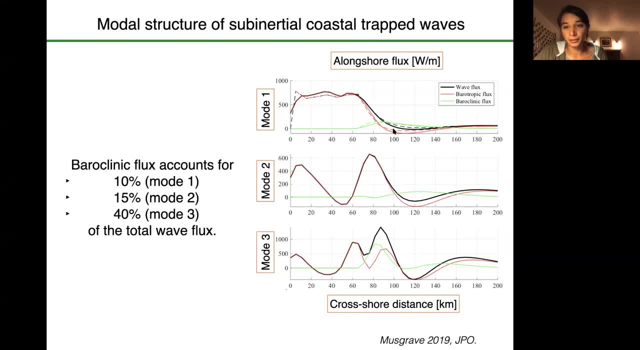 Over the shelf. that's this region here. once you reach the sloping region of the shelf break, then you start to acquire a baroclinic component. And if you go off and you only calculate the baroclinic flux from a mooring or from a model, then you will be severely underestimating the 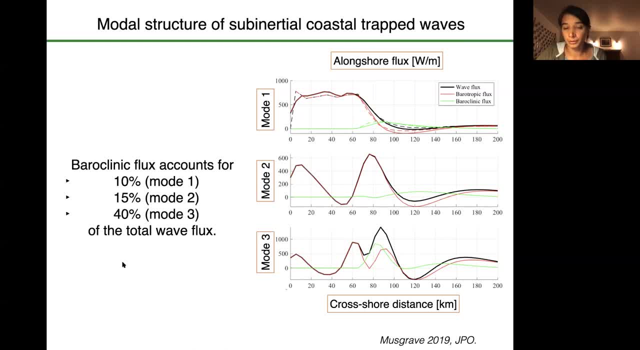 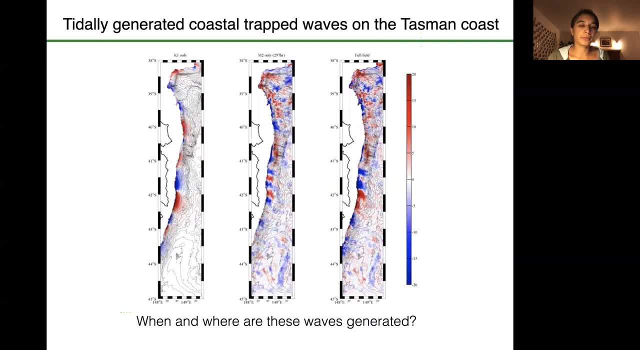 total flux in the wave And these are some estimates for this particular case. So that's a little bit of theory and a little bit of background. So the question is, do we ever see these waves anywhere in the ocean? And, as I mentioned, it's hard to really observe them. There have definitely been observations of 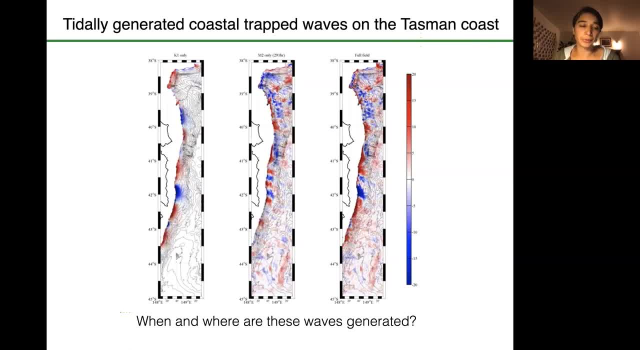 subinertial internal tides. both at the Mendocino Ridge and other places St Kilda in Northern Scotland, there has been evidence of these things. Superinertial trapped waves much less so. However, there are numerical models, such as the one that I'm showing here, that suggest that these 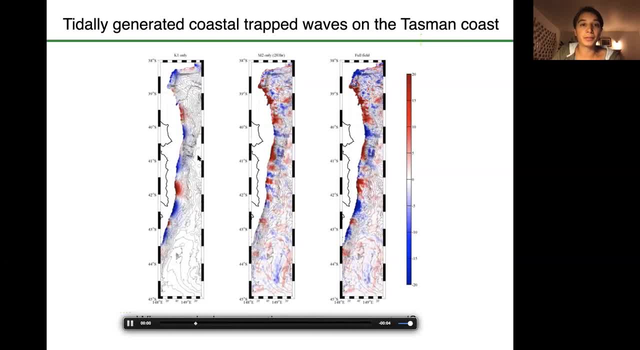 things might exist, even if they are hard to measure. So this is a numerical simulation of waves on the Tasman coast And what I've done here this is: I forced it with the barotropic tide at the boundaries and I'm looking at the interior response And what you're looking at. 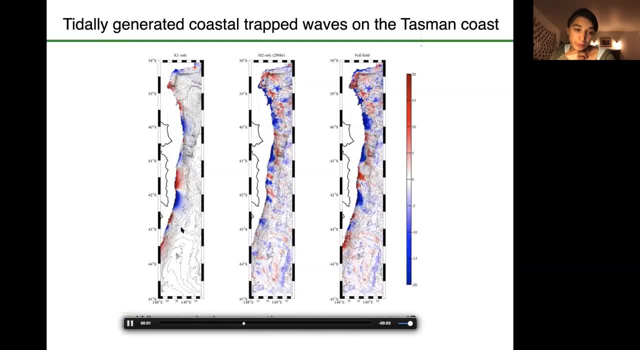 in color. here is the vertical displacements of an isopignol, of a given isopignol, And I've decomposed a time series of waves to extract only the subinertial component here. So this is the K1 constituent here. 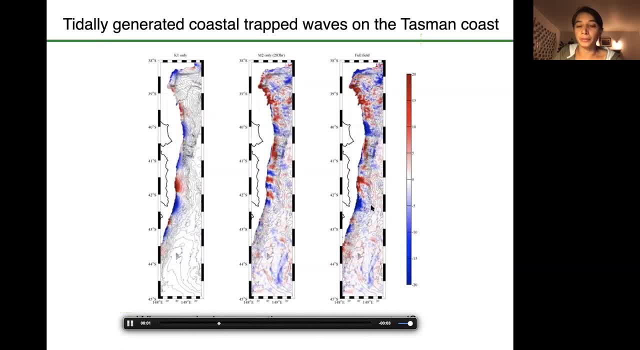 and the superinertial, the M2 constituent here And then on the far right, this is the full field, So you can see these fully trapped subinertial waves propagating up the coast, And what was kind of surprising, looking at this, is that there is evidence of these. 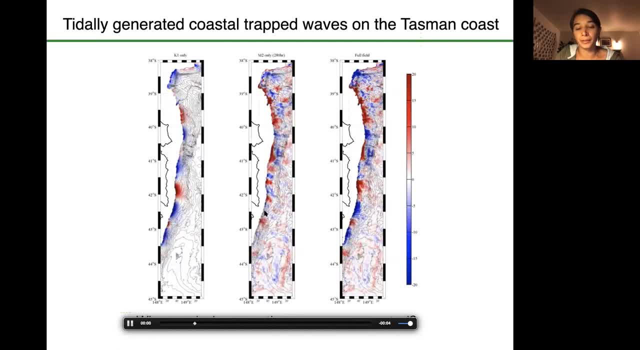 superinertial trapped waves also propagating up the coast, at least in this region here. So the question I'm going to try and get to with the last part of this talk is: under what circumstances can we generate these waves, What conditions And how likely is it that we expect to see them? 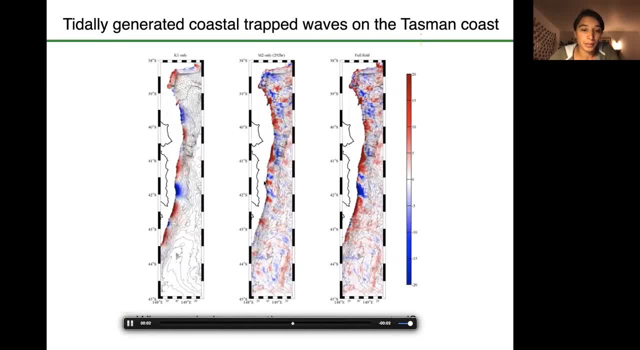 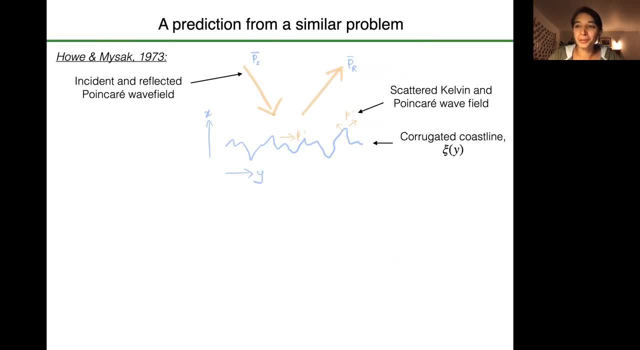 in the real ocean, And so, as with almost everything in this field, someone has thought about this problem before, or at least a very similar problem, And so the similar problem is this: how, in MISAAC in 1973, considered a homogeneous or an unstratified ocean 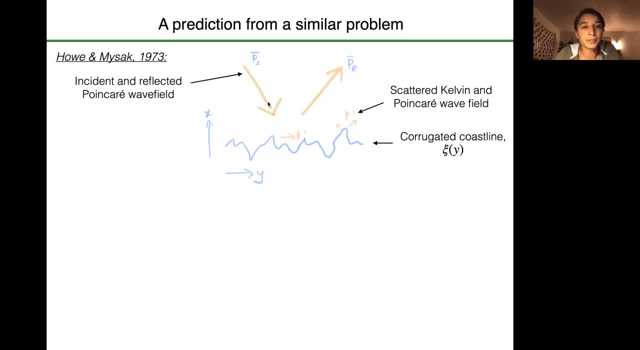 and the interaction of an incident- Poincare wave- that comes in towards the coast and reflects from the coast and the coast has some corrugations in it that I'm indicating with xe, which is a function of y, the long shelf distance, And what they found was that that incident 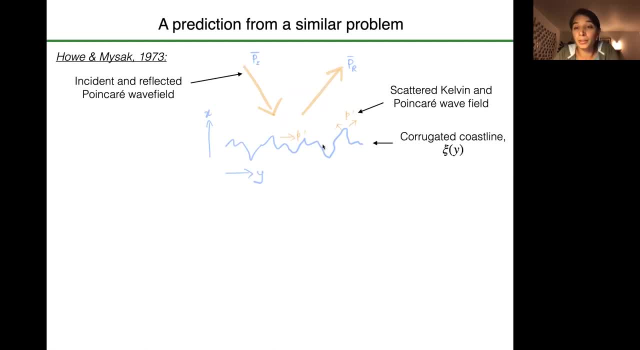 that incident, energy can scatter into kelvin waves. so kelvin waves are the allowable waves on a vertical, in a homogeneous ocean, along along a vertical wall with no, with no profile, and essentially so. this is the the set of equations that they solved. it looks somewhat like this, the set of equations that i wrote down before. they're assuming a pressure field. 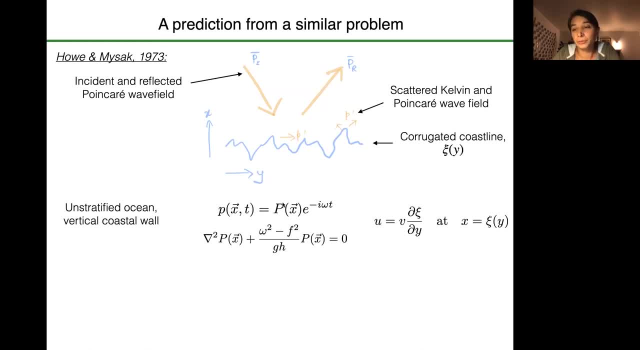 which is a function of space and time. they decompose it into a spatial mode and and they assume a solution that is has the frequency of the incident, the incident wave, and they come up with a governing equation. the key part here is the boundary condition. so the boundary condition 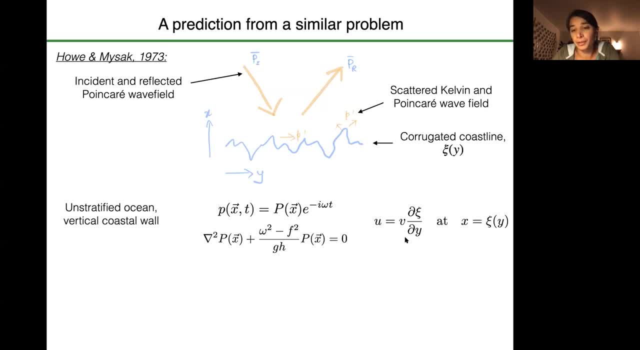 that they're imposing is that there's no flow through the boundary, and so you can see. well, let me skip to the result, and then i'll i'll explain you how this comes about and what they find, which i actually think is pretty, pretty cool. um so what? 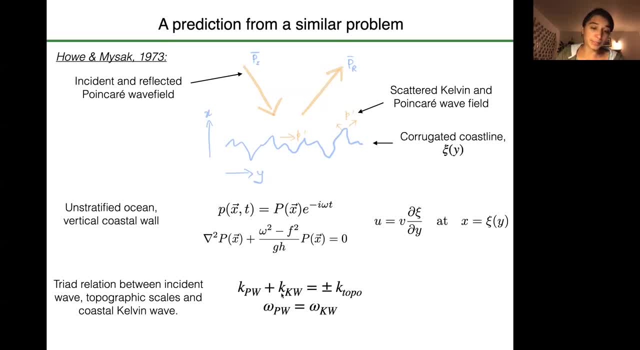 they find is that um energy is scattered into um a kelvin wave and a long shelf propagating kelvin wave, when the incident ponkari wave and the topographic scales satisfy this triad relation. and so um. for those of you who are familiar with wave wave wave interactions in the ocean, this is: 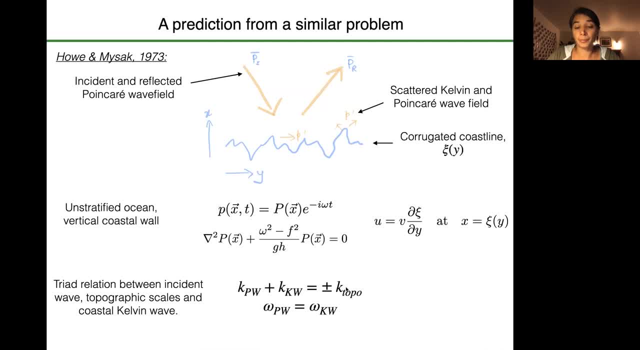 basically exactly the same thing that's going on here. um, what's happening is that for wave wave interactions, you have, um, a non-linear interaction that arises from the, the quadratic non-linearity in the, in the navier-stokes equation, um and when, um, and so if you have two waves, uh, in that quadratic non-linearity that the exponents add, 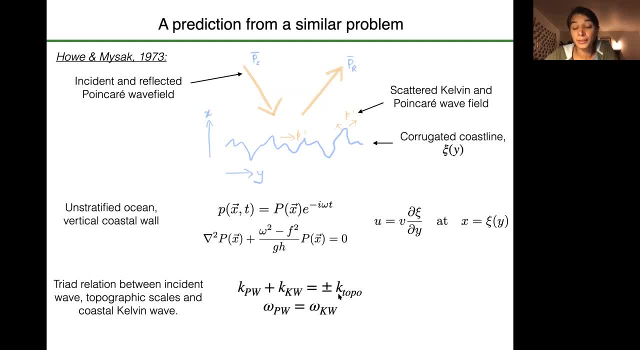 together, and if the sum of the exponents uh satisfies the dispersion curve um of a free wave, throughcipt, Give x, this-cylinder um of a free wave and the using this wave, then this acts as like a resonant forcing to the system of equations um, and so the analogous thing that's happening here. so we 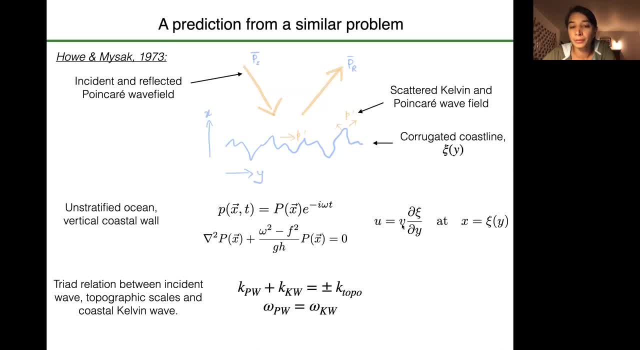 don't have any non-linearities in the governing equation, but we have this, um apparent non-linearity in the boundary condition, and so we have a correlation between the um, the long shelf currents and the scales of the bathymetry. and so what's happening is the bathymetry is acting like um, like pessoave, like 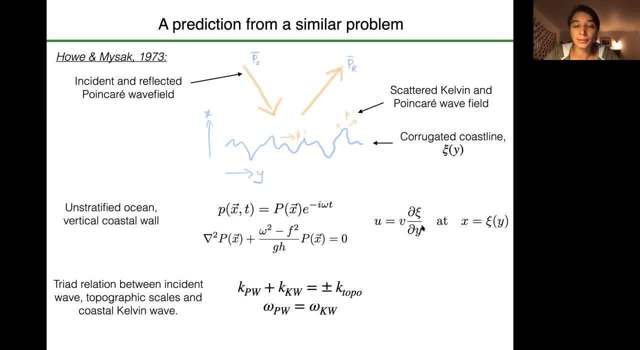 interact with the incident-poincare waves such that energy is scattered into a third wave And in this case, in the Howe and Misak case, that was a Kelvin wave. So this gives us an indication of when we might expect this to happen in a stratified ocean. 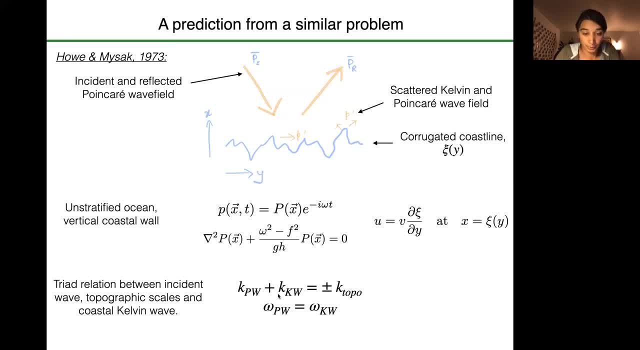 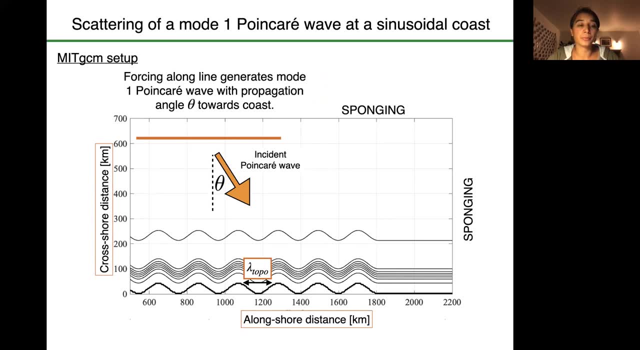 when we have a real cross-shelf profile, And so that's what I'm going to explore with a series of simulations now that I want to show you. And so what we did here was we configured the MIT GCM, a numerical model, so that we can essentially shine an incident-poincare wave. 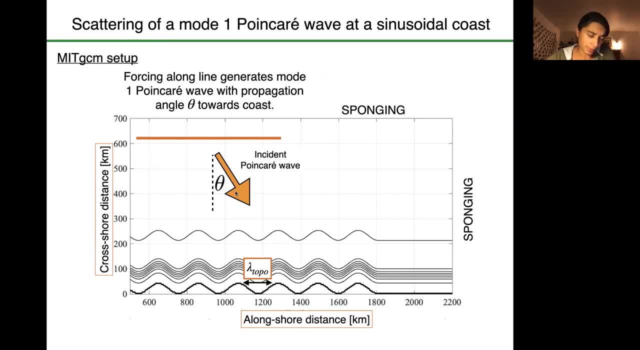 onto the coast, And so we adjust the angle of incidence of the poincare wave, So we adjust this angle, theta, And we adjust the corrugations, the length scale of the topography, And essentially we're looking for some combination of the incident, the angle of incidence of the incident. 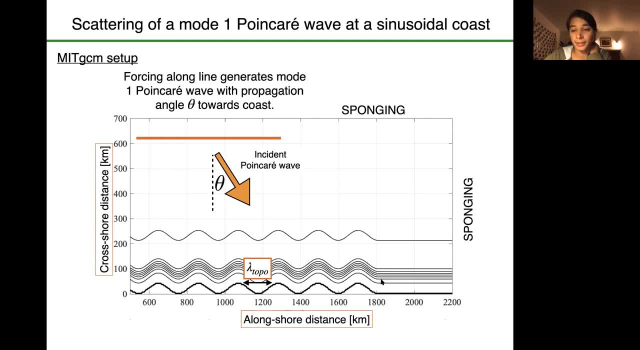 poincare wave with the topographic length scale such that energy is scattered into these coastal trap waves, And so you'll notice, as I change theta, I'm not changing the absolute wavelength of the incident wave, but I am changing the projection of that wavelength along the shelf. 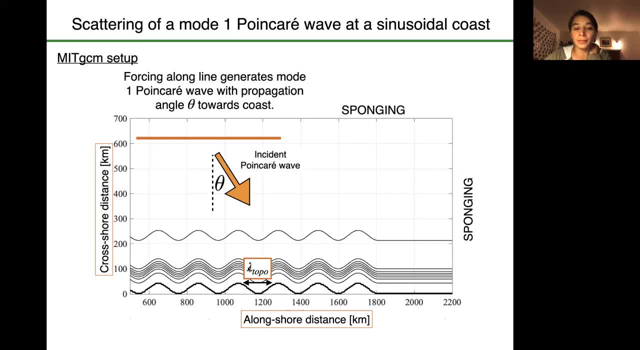 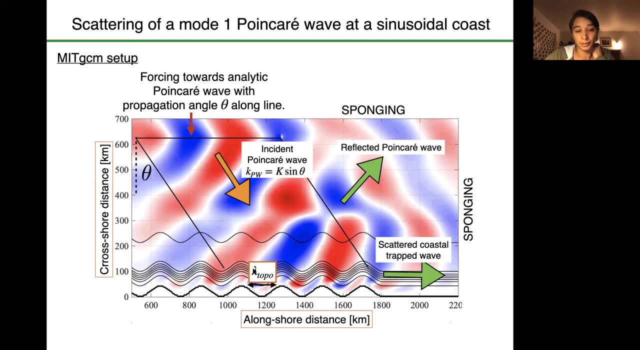 And so in that sense, even for a fixed wavelength, I'm changing the apparent wavelength of the incident wave such that we might hit resonance, And so here's a snapshot of what the flow looks like for a particular theta and a particular lambda toco that I chose, And I think this is. 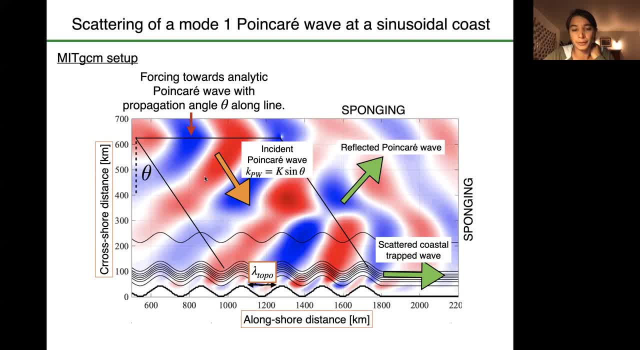 surface u or surface v. It's one of the components of the velocity, And so you can see that the incident wave field is propagating down towards the shelf and then it reflects. There's the reflected poincare wave that you can see out here. 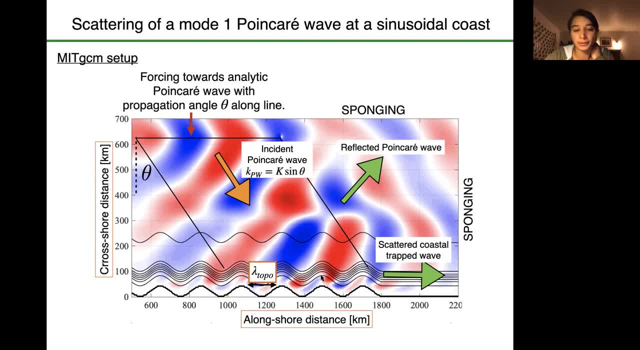 Then something's happening over these corrugations. You can see the formation of these kind of smaller waves, And so this is a resonant case, And what we're seeing here is the formation of a scattered coastal trap wave. And so to measure what I'm going to do, is I'm going to 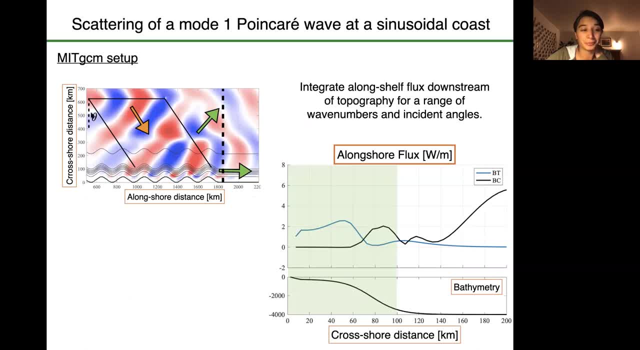 run this simulation a lot of times for a range of theses and for a range of different topographic length scales, And I'm going to look at how much energy is scattered into this coastal trap wave by measuring the flux just downstream to the right of the corrugations. So here's an example of what 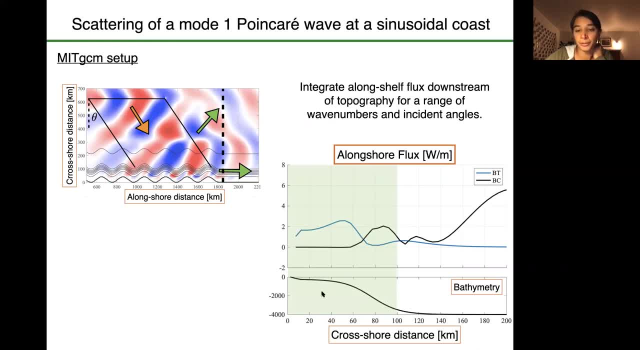 the flux looks like for this particular simulation. Here's the bathymetric profile. This is along this dashed line here And this is the alongshore flux in the barotropic and the baroclinic, in the blue and the black, And I'm just going to integrate the alongshore flux over this region. 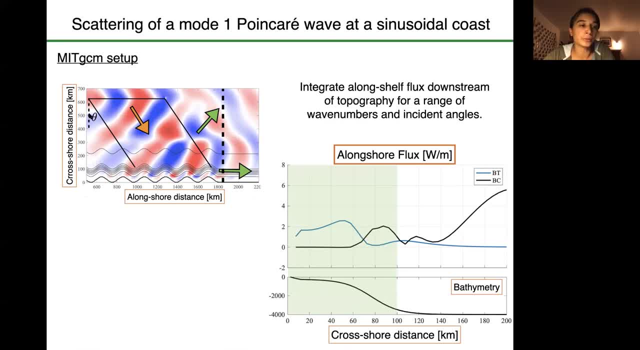 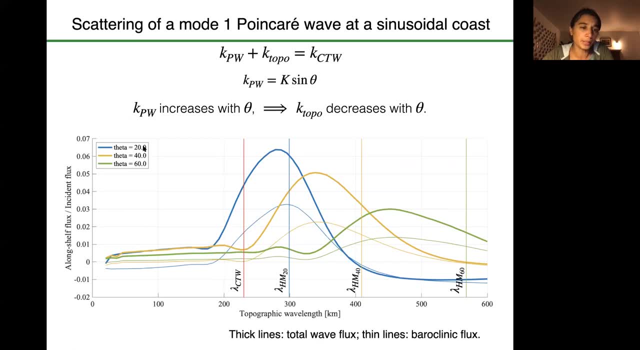 and I'm going to measure that. That's going to be my metric as to whether or not there's resonance for a range of theta and a range of lambda, And this is what I end up with. So this is for three different theses. So theta is 20 degrees, So that means that it's. 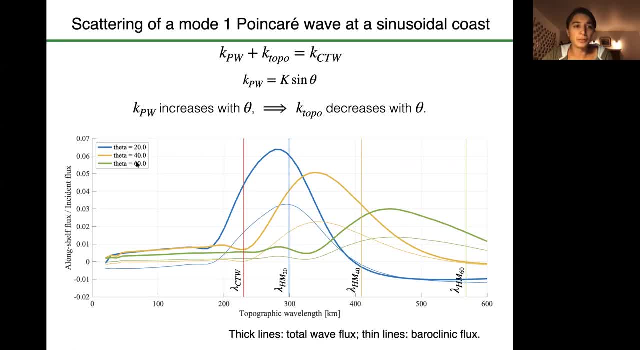 very nearly normally incident, And when theta is 60, it's more oblique, And so when it's almost normally incident, we do actually see an increase in the flux, in the alongshore flux, when the topographic wavelength has scales of around about 280 kilometers. I've normalized this alongshore flux by the incident. 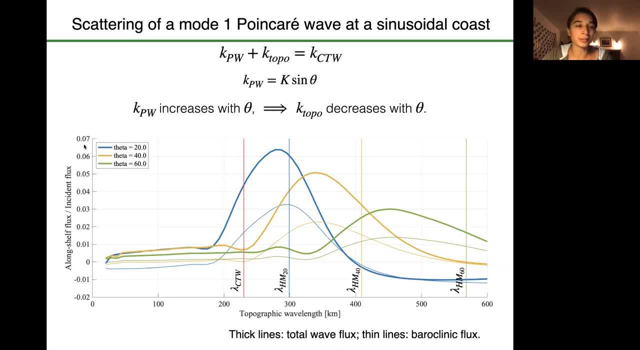 flux. So this gives you a sense of how much energy we're talking about here. So it's not tons, you know. seven percent, This is very much a ballpark figure, but you know, it's not all of the energy by any stretch, It's not even most of it. Nevertheless, we are qualitatively seeing. 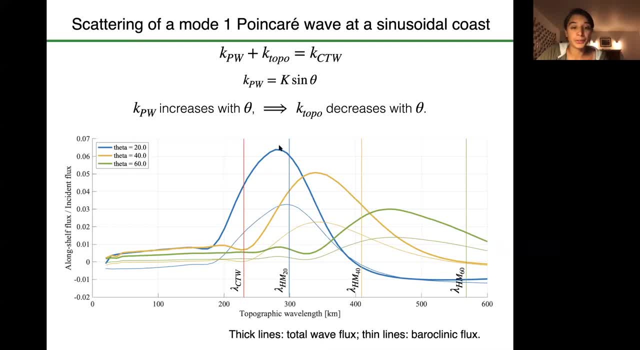 the behavior that we would expect from the Howe and Misak theory. So we see, as the projected wavelength at the shelf decreases, So as we increase theta, that projected wavelength at the coast increases, sorry, decreases. We see the resonant wavelength. 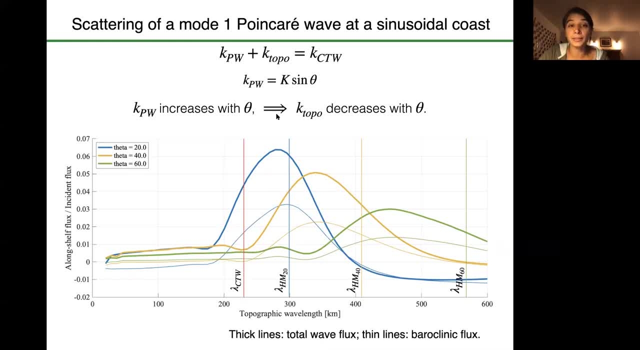 the topographic wavelength shifts to larger and larger scales And this is consistent with this triad relation. For reference, I put the Howe and Misak predictions on here. We wouldn't really expect them to match. We wouldn't expect them to match. We wouldn't expect them to match the 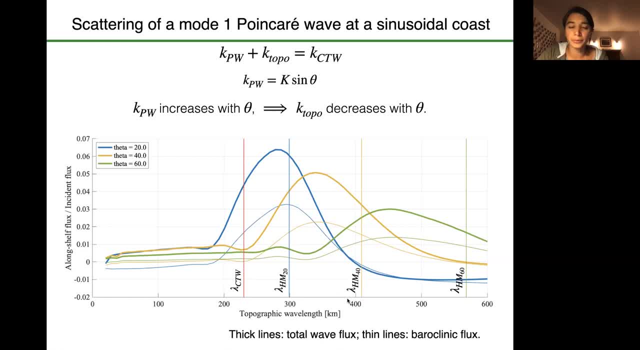 anyway, because they were working in a homogeneous ocean with a vertical wall, But you can see how the quantitative behavior from their predictions is satisfied here as well. So this addresses how superinertial internal tides can be generated at the coast by the scattering from an incident internal tide. So what about subinertial internal? 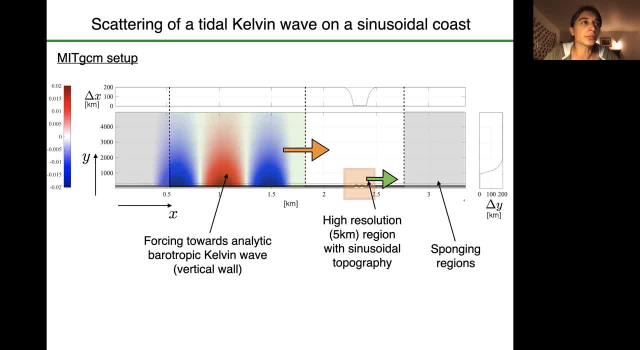 tides at the coast. So obviously you can't generate a subinertial coastal trap wave from an incident Poincaré wave, because those Poincaré waves can't exist at subinertial frequencies And so the only mechanism is scattering from a lower mode coastal trap wave. 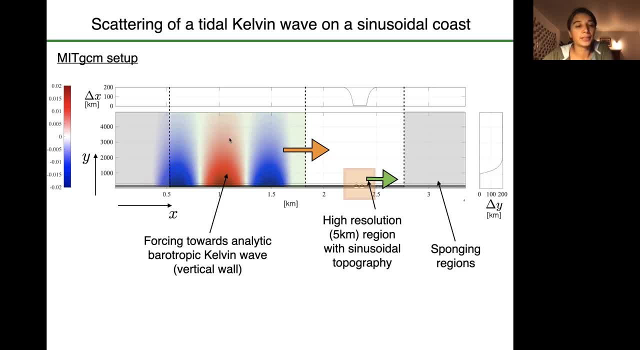 essentially a Kelvin wave in this case. So this is something. so what I'm doing here is I'm forcing the model towards something like the Graebus-Kelvin wave, which is something like the tide that propagates along the coast, And so I force it towards that and I let 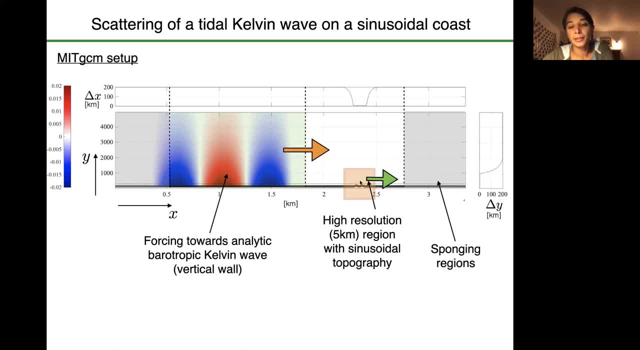 that wave propagate out of the domain and then it interacts with this region of topography. So in this problem there's no angle to change. The only parameter that I can change here is the length scale of the topography, And then we can assess how much energy is scattered into. 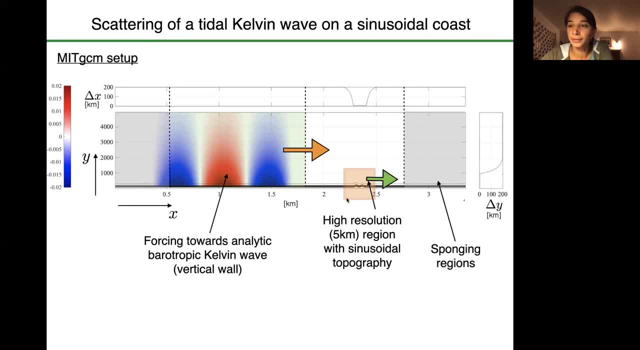 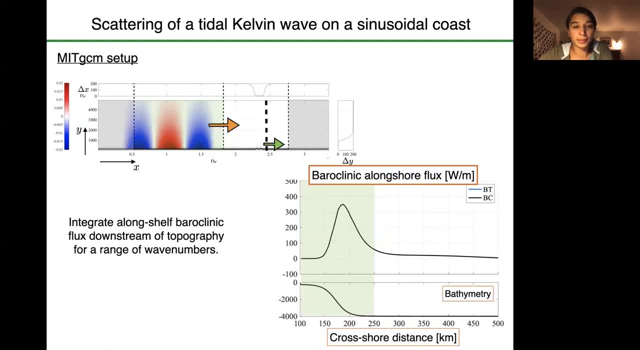 coastal trap waves, depending on the length scale of this topography for a given time. And I can also do this by doing an incident: Kelvin wave at a certain frequency, And so again, I'm going to do the same thing, I'm going to calculate the flux just downstream. 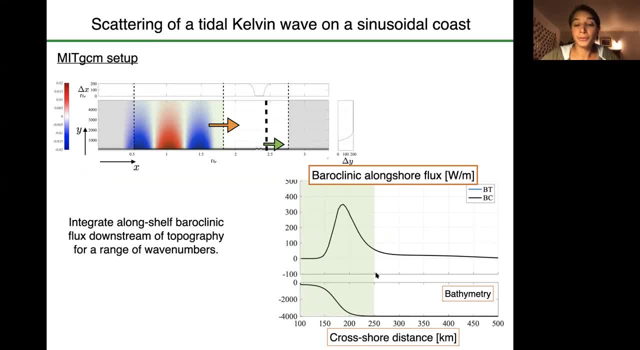 of the topography and I'm going to integrate it over some region. And for this I'm only looking at the baroclinic component of the alongshore flux, because it's very difficult to separate the barotropic component from the forcing wave itself, which has a large barotropic component. So this 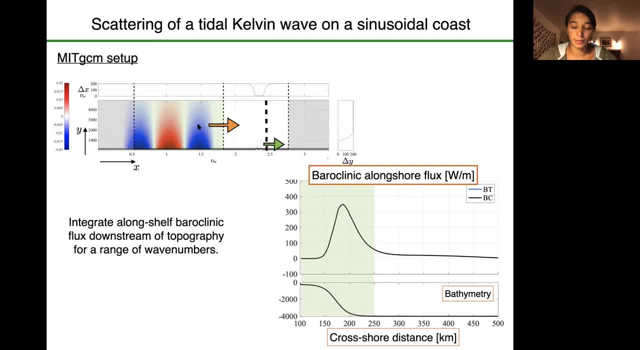 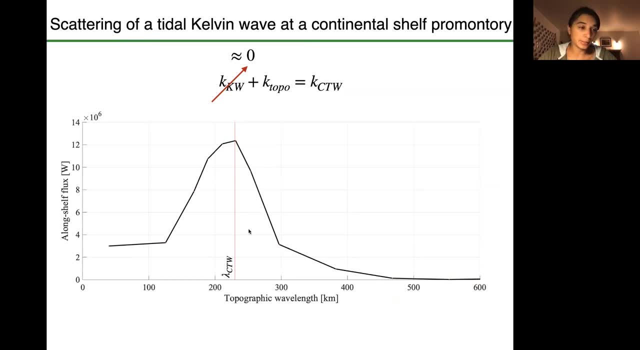 kind of goes back to this issue of how it can be hard to do energetics with these waves waves. But anyway, if I do this, I do it for a range of topographic wavelengths And indeed we do see a peak in the long-shell flux at a certain topographic wavelength. And again, 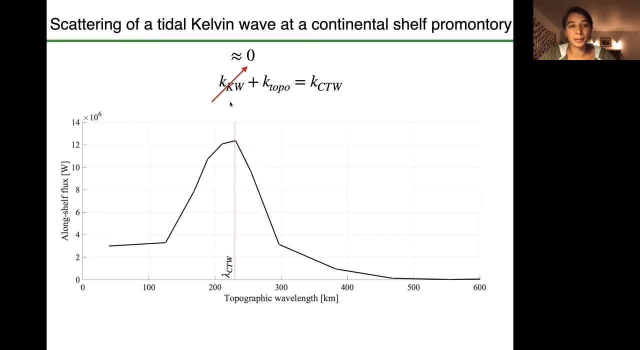 it seems to be largely in agreement with the Howe and Misak prediction, which is that when k-topo, when the wave number of topography is close to the wave number of the coastal trap wave, this is where we see this resonance, And it's basically because the wave number of 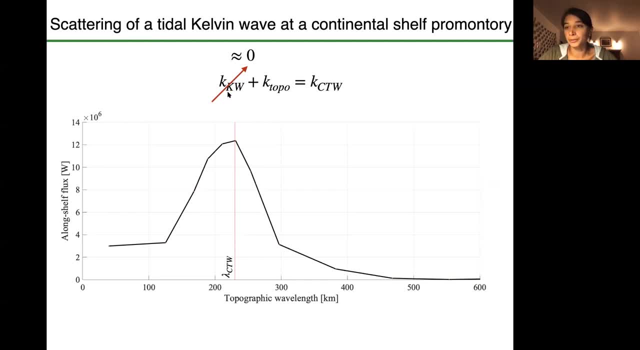 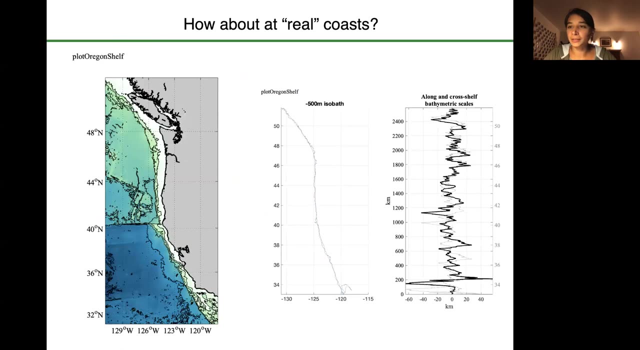 the generation Kelvin wave is very close to zero. It has very large scales, So there's two mechanisms in an idealized model as to how you can generate these things. Whether this happens in the real ocean is still an open question, but I can explore a little bit more deeply with 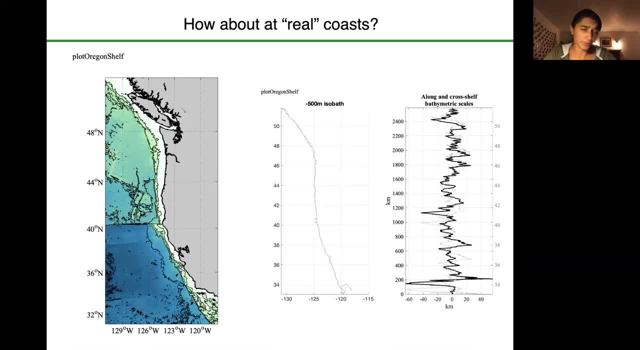 realistic models, And I'm going to show you a little bit of an example of this. So this is realistic bathymetry, And so that's what I'm going to show you next. So at real coasts. well, I'm going to construct my real coast by taking something like the west coast of the United. 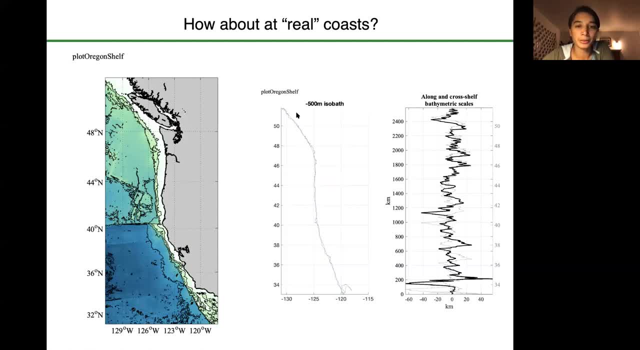 States, And I take the 500-meter isobath, And so that's what I plotted here. the function of this is longitude and latitude, And then I high pass it and I calculate the distances, And so this is what the coast looks like by the time I've done this. This was actually a 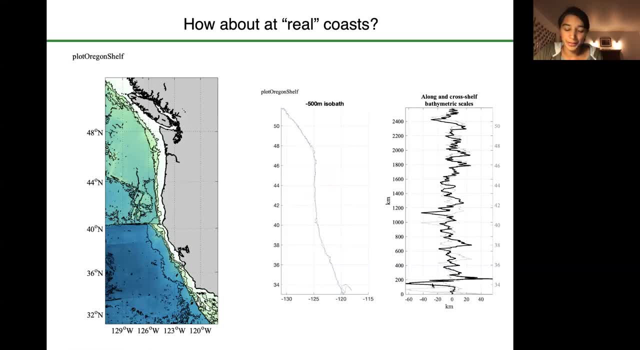 pretty interesting exercise for me. It wasn't obvious to me looking at this profile what the scales would be and how this would look, But it is interesting to note that there are some definite scales. I haven't actually made a spectrum of this profile, but you can see that. 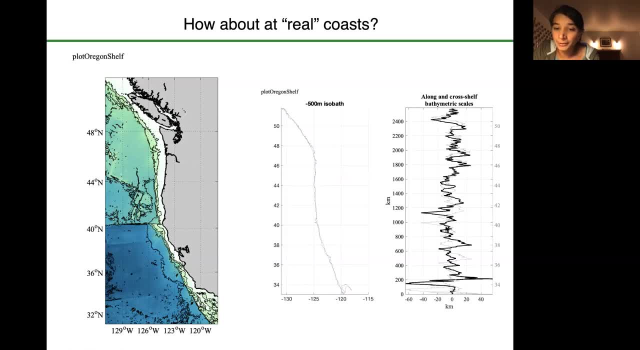 there are some definite scales here. So the long shelf corrugations do have scales of order: 100 kilometers or so. The amplitude of the corrugations, well, some are very large, 100 kilometers, Most are 20 kilometers or so, And actually, once you get north of the Mendocino Ridge, 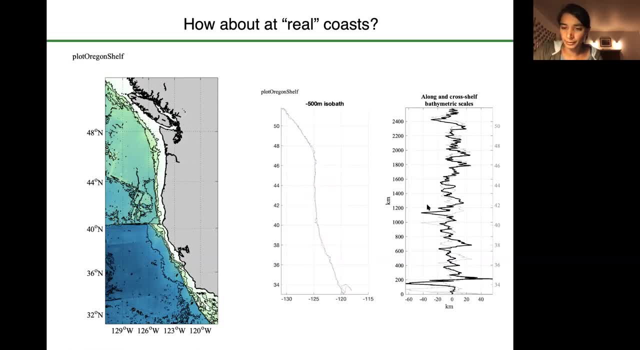 it seems like the spectrum really changes it And there are much smaller scales in there. I'm sure that some geophysicists would know what sets the long shelf scales here. If anyone has any ideas, I would be really interested to hear them, because they're very important to this. 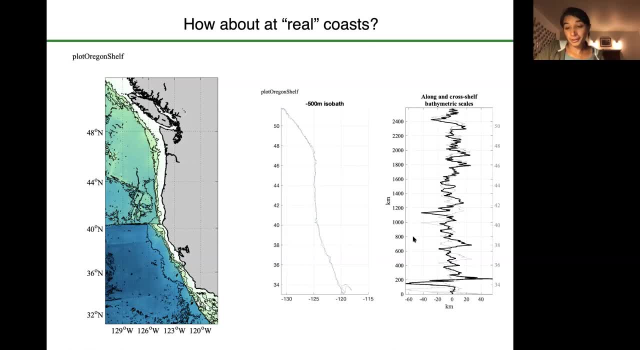 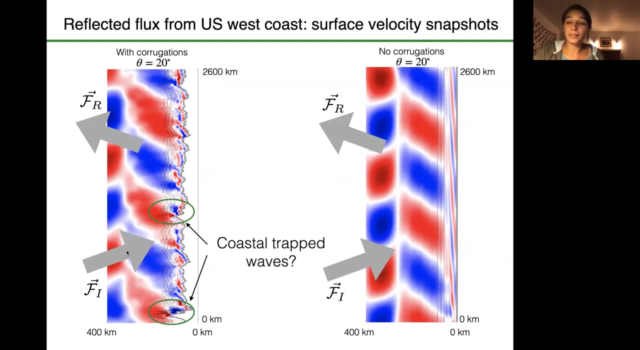 problem, as we will see. So what I'm going to do, I'm going to take my version of the west coast of the United States and I'm going to put that in my model, And then I'm going to shine a bunch of incident Planck-Array waves at the coast And I'm going to do it at a range of angles And 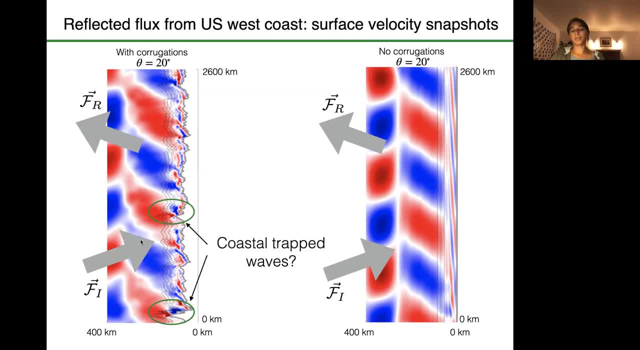 so these are some snapshots of the surface velocity for one of these simulations. So I chose an incident angle of 20 degrees to show you here, And so I have a kind of control run. It's a little bit difficult with the current, but I'm going to do it at a range of angles. So I'm going to 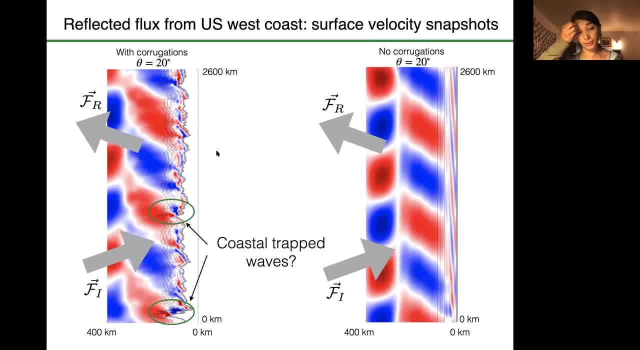 this model because there is viscosity in the model and so i wanted to um, i have a control run where i don't have corrugations, so that i can try and um back out what the influence of the corrugations are, and so, um, here's a snapshot. so, with 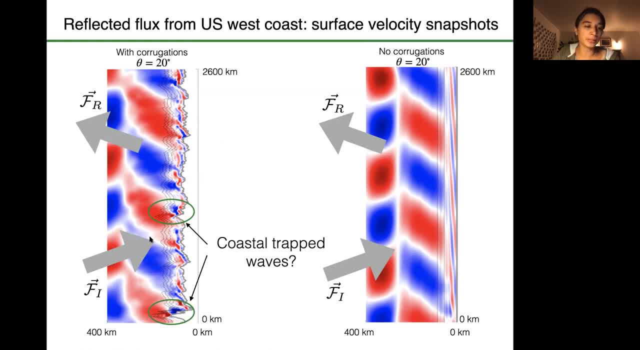 corrugations. you can see that the large scale pattern this is from the incident and reflected waves, but along the coast you can see, um, things that look somewhat reminiscent to the generation of coastal trap waves. um, um, at least they look, uh, much like that from the, the idealized simulations that i showed. 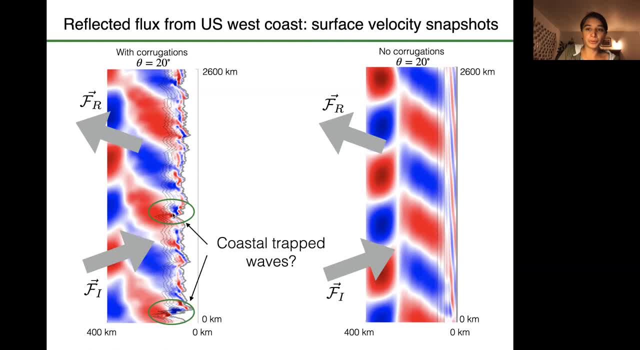 you earlier, um, but perhaps um, what is more striking is the generation of these stripes here. so these are, uh, these are um, small scale waves and in fact, uh, these are leaky edge waves and they've been discussed by chapman in in 1982 and clearly this is another, um, another, um phenomenon that the incident 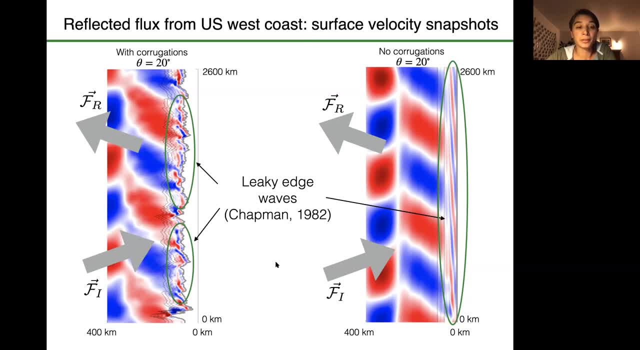 uh, the incident wave can scatter energy into um, at these edge waves, um and and interestingly, we also see the edge waves when there are no corrugations on the shelf as well, so they don't rely on the on the presence of these along shelf corrugations to generate the edge waves. 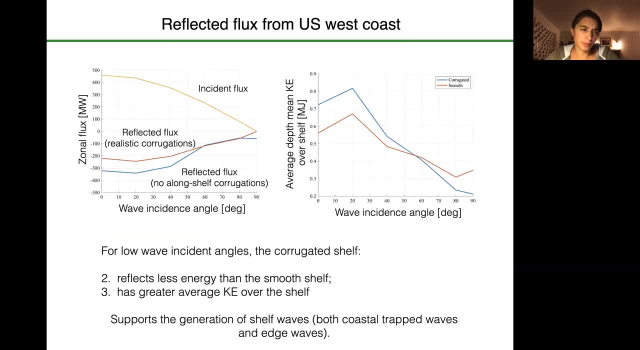 um, so um to, to summarize, so to summarize the output of these simulations, i i run um these at a range of incident, um, a range of incident angles, um, and, as i mentioned before, it's pretty hard to get at the energetics of these waves individually. 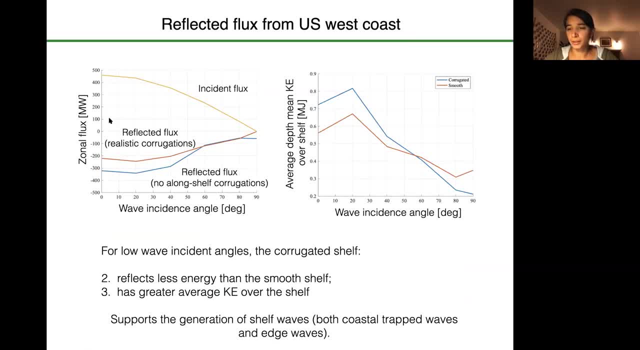 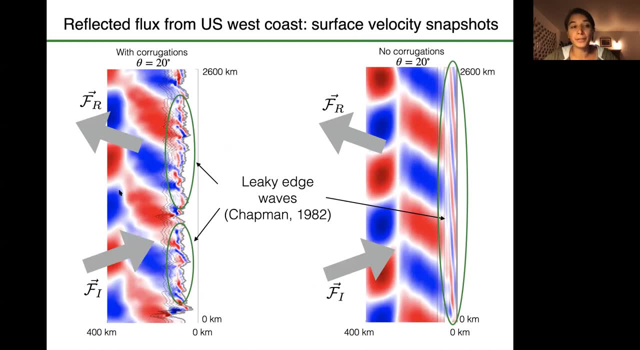 so i've been doing it from a kind of bulk view um. so what i do is i calculate the incident flux um in in this region, and then i just calculate the total reflected flux. and if the total reflected flux um is very much, uh less than the incident flux, then well, there must be some energy being lost at. 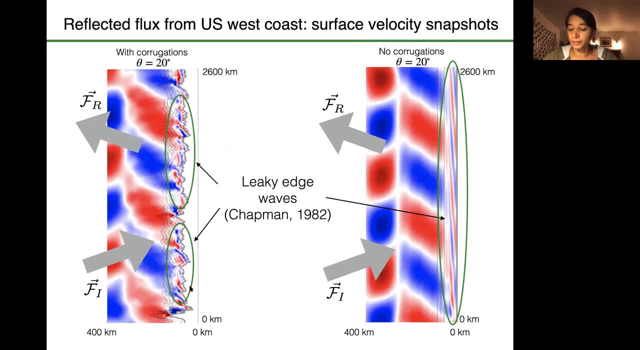 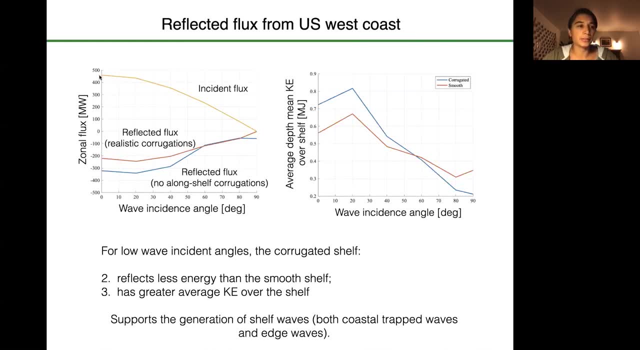 the shelf, and so i'm comparing how much energy is lost at the shelf, um as a function of different incident angles, um, and so that's that's what you're seeing here. so the incident flux as we um increase the angle, the incident flux goes down right when the wave is. 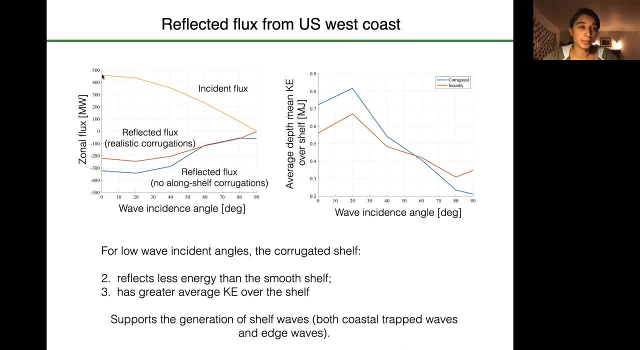 um is normally incident. we have maximum flux um incident shelf when the wave is parallel to the coast. then we don't have any incident flux um. so that makes sense, the reflected flux. well, um, first of all, consider the case where we have no along shelf corrugations, that's this blue line here. 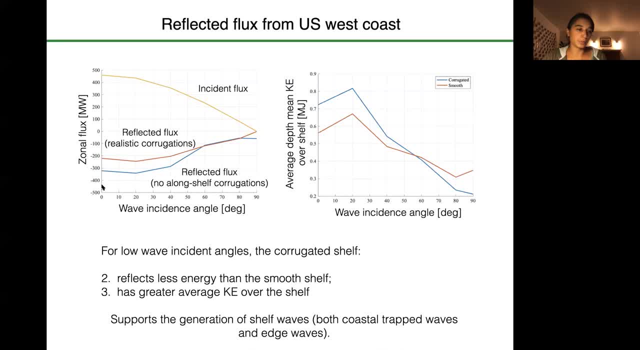 if there was no viscosity whatsoever, then i would expect that this would have the same action amplitude as the yellow line. everything would just be reflected straight off the shelf. but obviously there are some other things going on in the model and we are losing energy over the shelf. um, however, we are losing more energy. 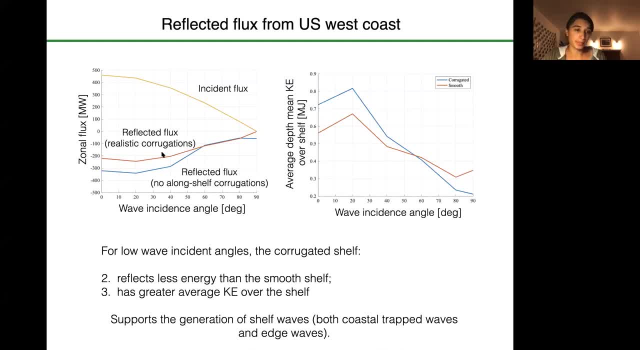 when we have these corrugations along the shelf. um, so energy is um being scattered to small scales, um, perhaps, uh, through the the generation of these coastal trap waves. um, and this is um another way to see, it's kind of consistent with that. that figure on the left is that the 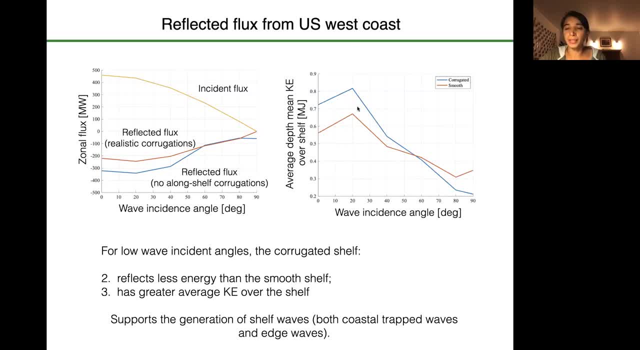 the, the mean kinetic energy um over the shelf break is actually um rather larger for uh, for closer to normally incident waves um than compared to the smooth case, and so energy is being scattered into motions, um over the shelf break, um, and it's concentrating kinetic energy over 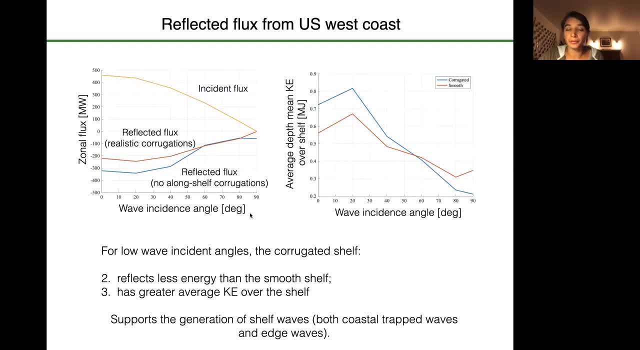 the shelf break at these small scales, which can be a precursor to mixing. so these simulations um a little bit preliminary, but they do support the generation of these shelf and actually highlight perhaps the importance of edge waves, in addition to the coastal trap waves that I've been talking about. Okay, so that's all. 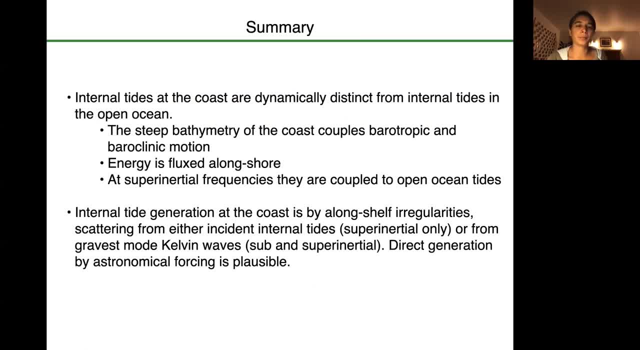 I have two points for my summary. So internal tides at the coast are pretty different to internal tides in the open ocean, and they're a little bit harder to work with. The reason is that the steep bathymetry of the coast couples together barotropic and baroclinic motions, and so this is kind of a 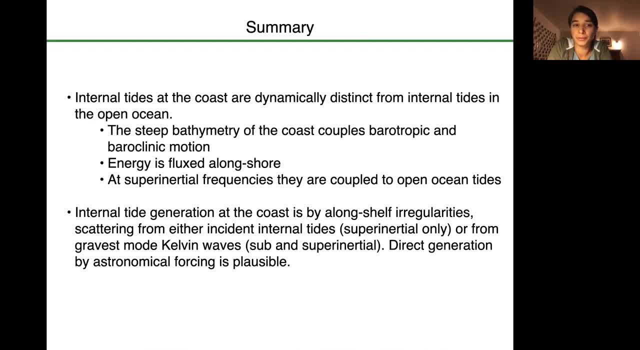 practical issue, but it does make it hard to separate the wave modes over the steep bathymetry. Energy is fluxed alongshore and it can't flux in any direction as it can in the open ocean And at super inertial frequencies. the wave modes themselves are coupled to the open ocean mode so they can exchange. 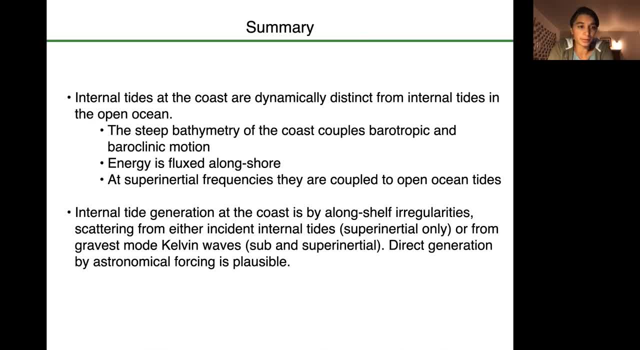 energy backwards and forwards. And then, second, there are two mechanisms by which we can generate these coastal trap waves. At super inertial frequencies they can be generated by scattering of an instant Pankare wave off of a long-shelf corrugations And at sub inertial and 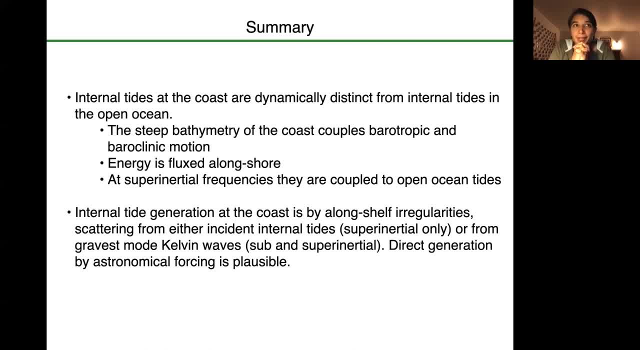 then the impact of an instant Kelvin wave with corrugation, so, for example, the barotropic tide as it propagates around the ocean basin and can also scatter into coastal trap waves at both sub and super inertial frequencies. The final point is that it seems plausible that the coastal trap 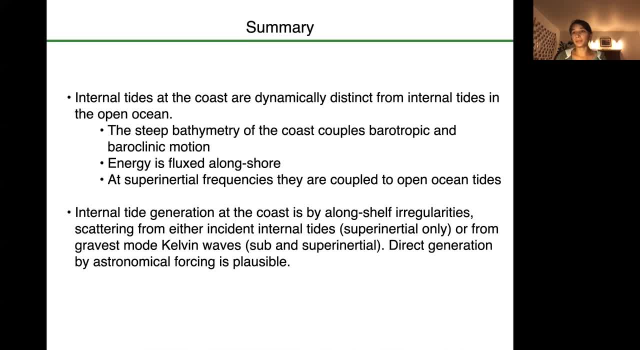 waves could be directly generated by astronomical forcing because they have a large barotropic component. so that kind of canonical energy pathway of you know, astronomical energy being transferred to the barotropic tide and then from the barotropic tide into internal tides, may not apply very well at the coast. 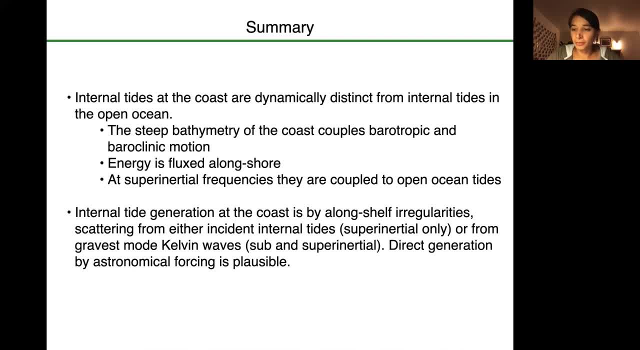 And so that is all that I have, and I'd be happy to take any questions if there are any. Thank you very much, and there won't be much applause which you won't get to hear, sorry. So, Navid, you're on. I'll let you manage the questions if you'd like to. there's nothing yet. 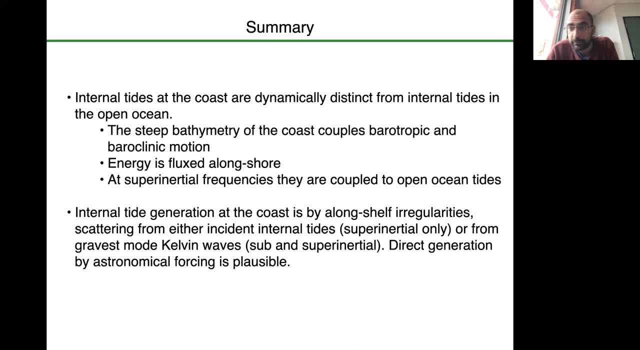 You can. you know people can unmute and ask questions. Okay, thank you very much. I may start with one. I don't see anything in the chat, So essentially here you showed another mechanism for energy for you know, for 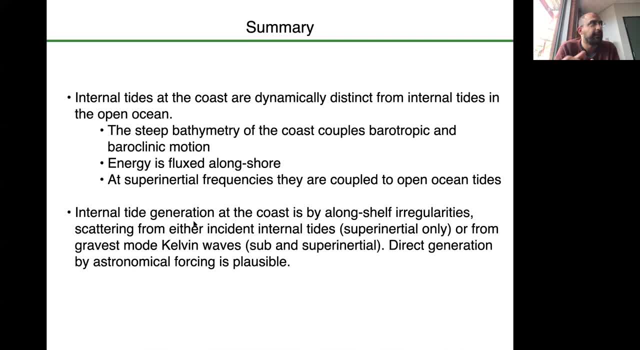 internal tides to be propagating or generated outside this. you know 30 degrees, you know like cutoff And this Gamma image gives you, you know, that digitalized grid pattern that we usually wait for the time that we are curating. 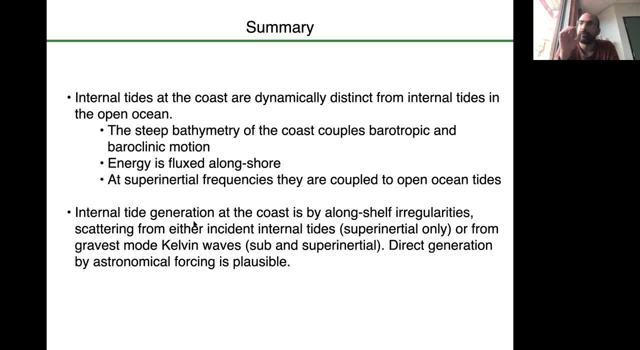 Exactly The ideal type of climate molecular measures that we usually think of when we're thinking of just generation of linear internal tides. So, and what you are arguing also is that you know if you are close to the coast because of this, because of bathymetry and the ability of the bathymeter to generate modes, even when you are, you know at latitudes that you wouldn't expect to see them: the barotropic tide and theta. 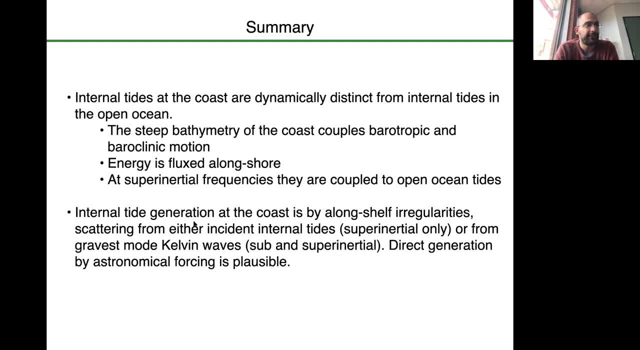 Okay, will can generate internal tides there and then they can propagate down outside. yeah, they can't, so I they don't have the freedom to propagate anywhere in the ocean. they can only propagate along the shelf. but but as they propagate along the shelf, they they can lead to dissipation. I mean, they will dissipate. 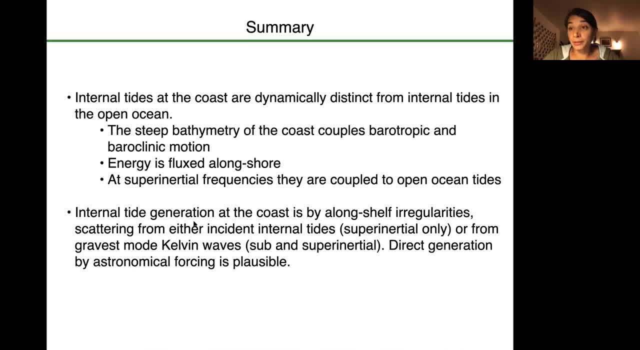 and they can lead to mixing deep along the shelf break. so and then you, you were, you were also saying: but now, because these are not purely baroclinic modes, it's very harder to distinguish when you're going out with a ship and you're measuring something you don't, you cannot say, ah, I'll take out my depth average of. 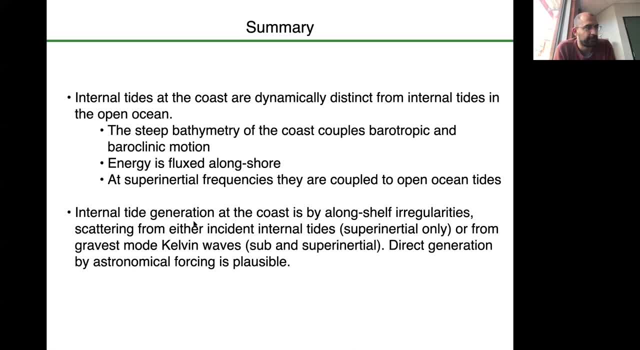 the flow, and the rest is about clinic flow and that's. you know, whatever it's in the frequency of the tide or whatever tide I'm expecting to have here, so so, but if you do your, you know, if you do your, you know, somehow you can do your. 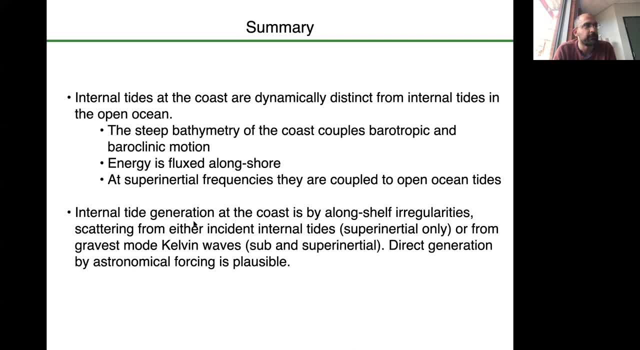 decomposition. can you then project to these modes that you get out of the analysis and and and then see how much of the flow is? you know, you know, you know you can do your decomposition, you can do your decomposition, these coastal internal tides, Yeah, so I think that that is the right way to do it. 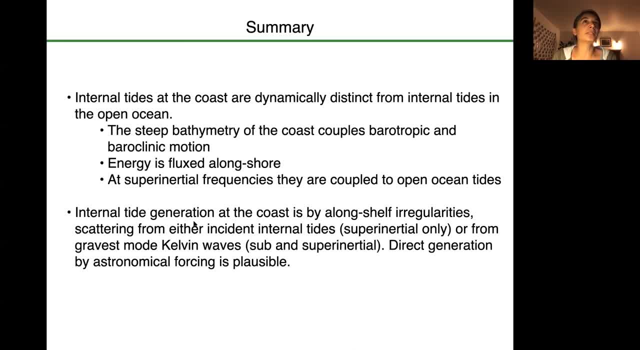 And you can formally do it. It is formally correct to do it in the long wave limit But unfortunately for short waves, which we're often talking about for tides, because they have slightly higher frequencies, the modes aren't orthogonal, which means that you can't really project directly. 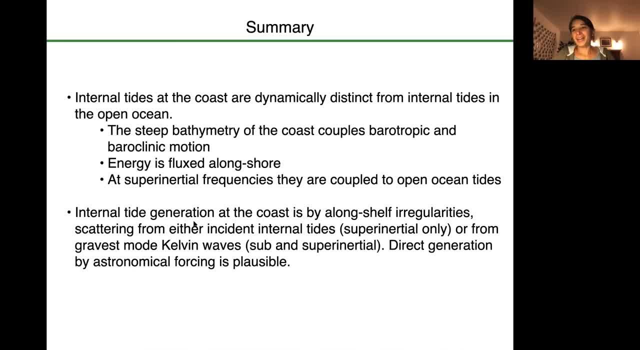 onto the modes. It's questionable. I mean the modes. they're solutions to the eigenmode problem, but they are not orthogonal. There's no orthogonality relation Like the bathymetry. it's like having a mean flow somehow. 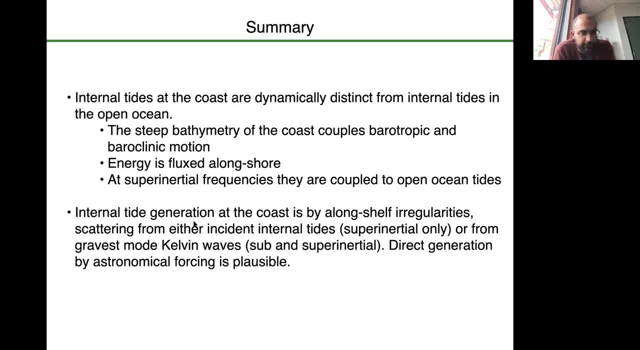 that mixes up everything together. Perhaps we're getting into the nitty gritty now. Huh, I haven't thought of it as being like a mean flow. Somehow it introduces no normality to the linear operator, But perhaps we can talk about it. 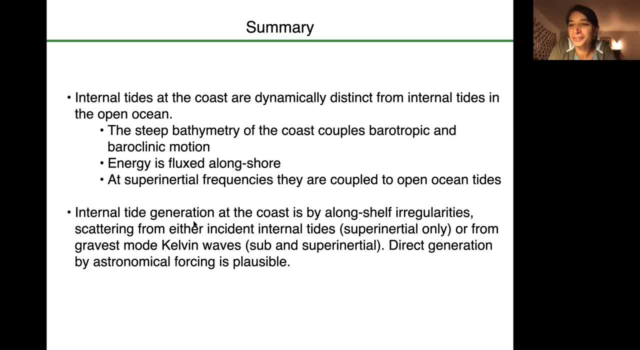 Huh, Yeah. Yeah, that sounds interesting. There are lots of analogies. There are lots of analogies across in wave behavior. I mean this analogy between wave-wave interaction and wave scattering. I find pretty interesting, Interesting indeed. Yeah, that was interesting. 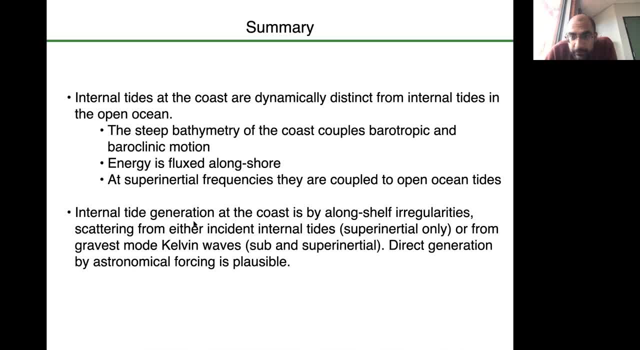 So yeah, Well, if there's no one else, I'll just ask a little bit about that tectonics question that you've raised about the. you know, basically I looked at that as there was a young versus old right. 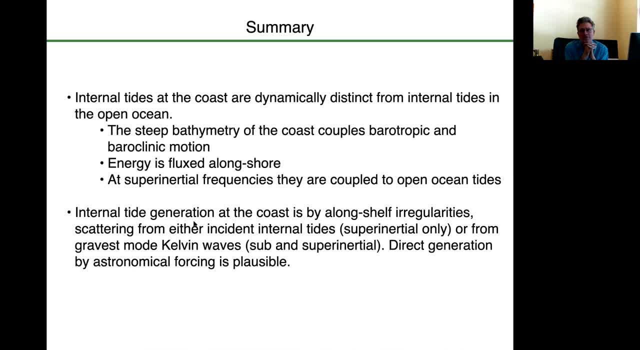 I mean, It's a very, very young seafloor north of the ridge, But I wonder, what is it that's the characteristic of that seafloor, or the coastline, or whatever it is that is driving the mode, you see, I mean, what would the change in? what is it you're looking for? 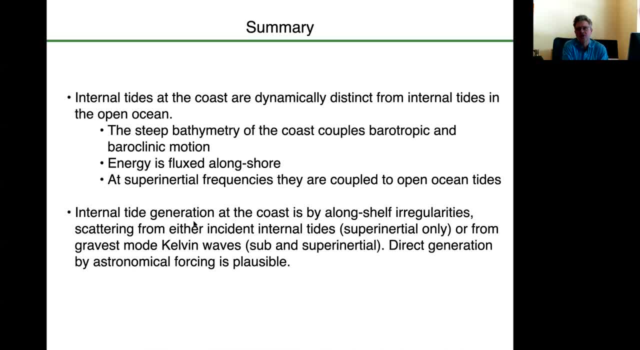 Are you looking for a change in the frequency content of the symmetry going north-south? Is that what it was? Yeah, I mean, I guess before I did it I had no idea what the length scales, what length scales I should expect to see in the coastline. 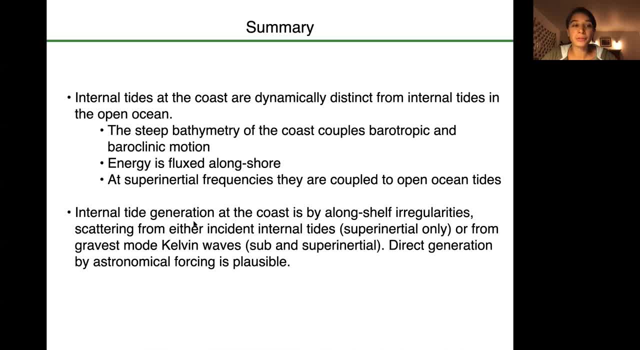 You know what is the spectrum of the coastline, And so when I did it, I can see that you know. it does seem like there are some predominant scales. I haven't made a spectrum, like I said, But I bet you, if I did, I'd see a peak at around about 100. 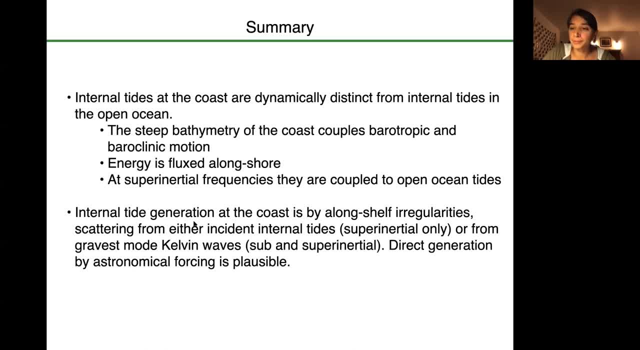 kilometers. It's very interesting, But there was like a sharp transition. right Yeah, Is this the US-Canada border there? What is that there? I thought it was the fracture zone. right, It's the transition from the strike motion to the seduction zones.